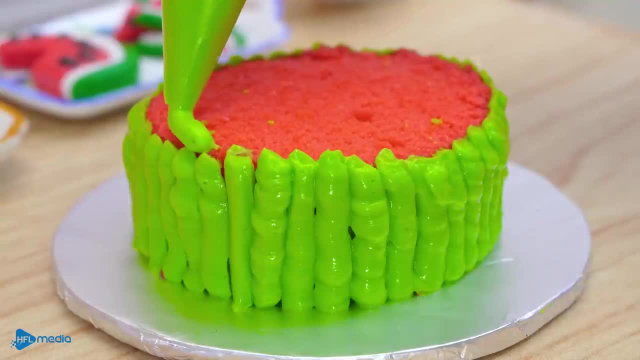 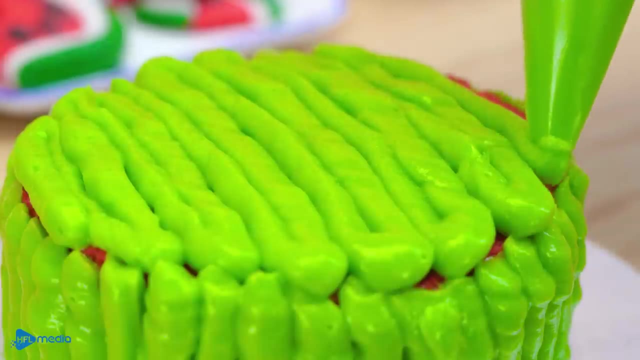 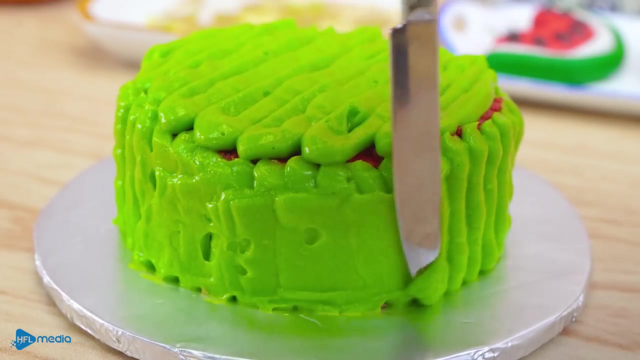 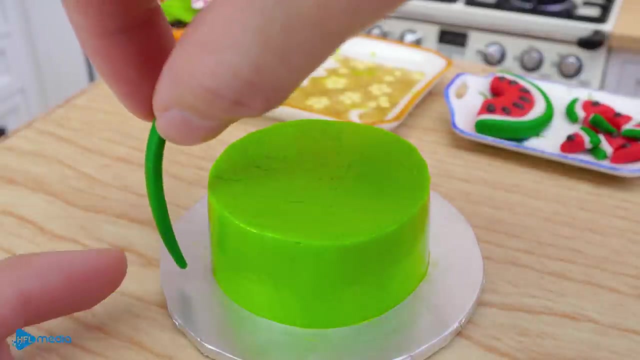 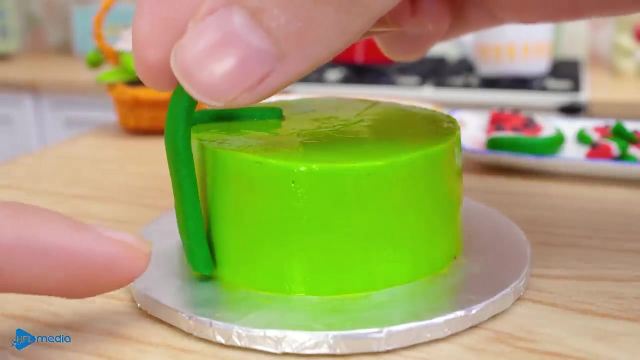 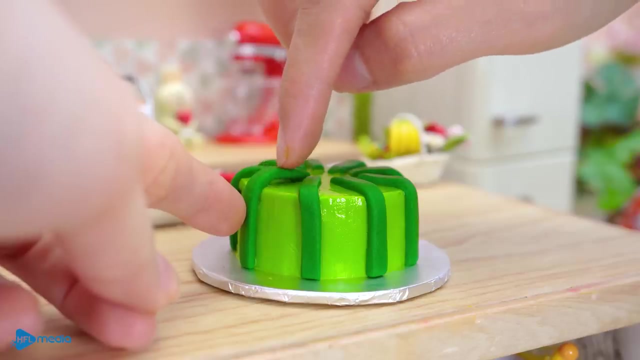 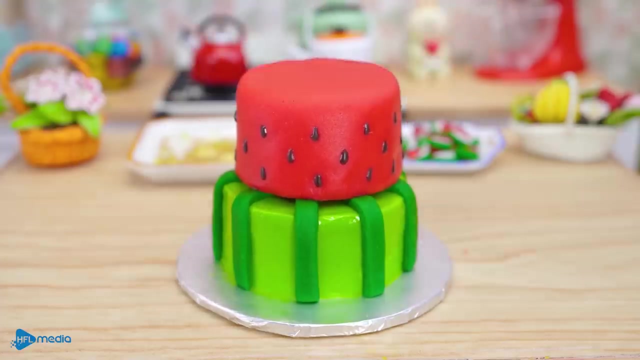 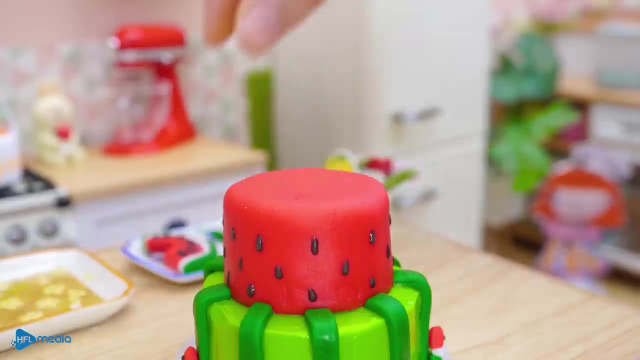 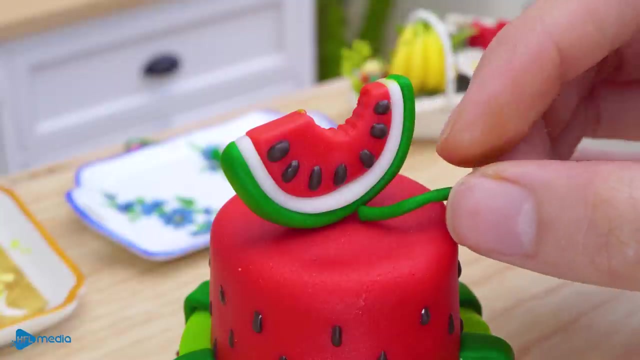 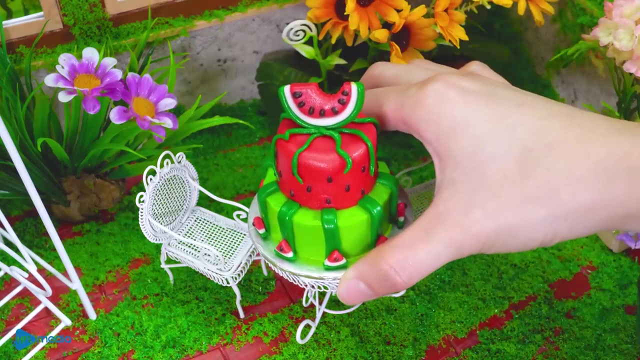 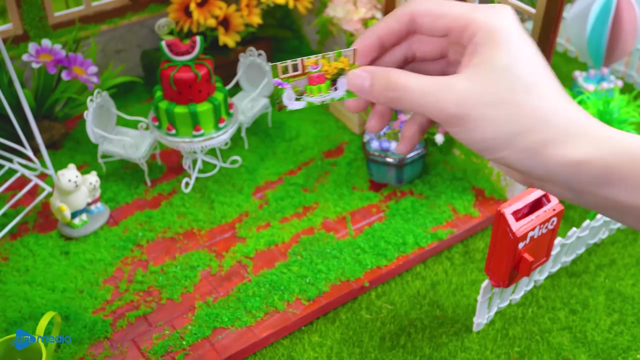 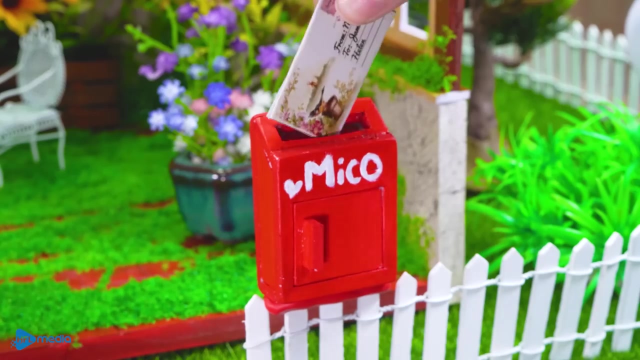 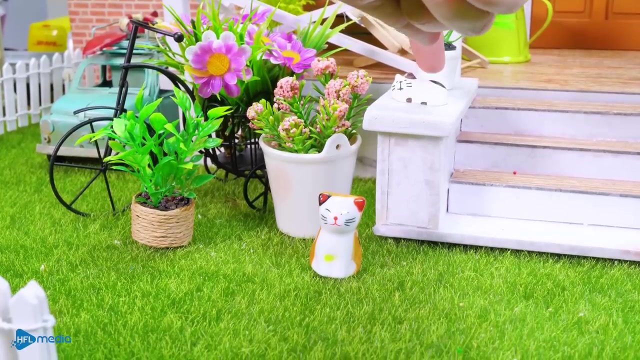 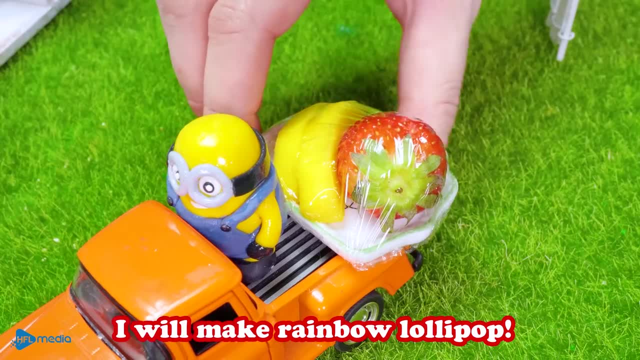 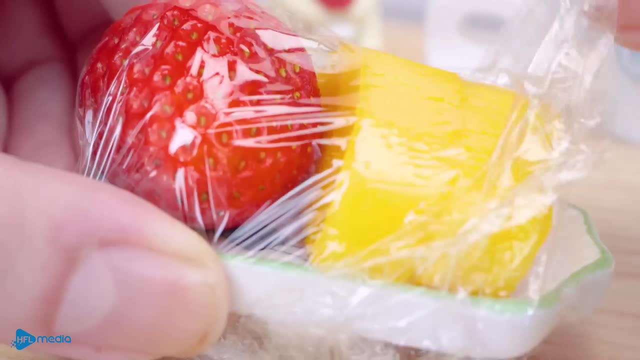 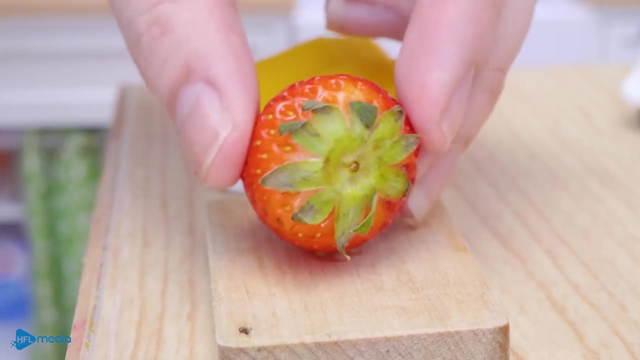 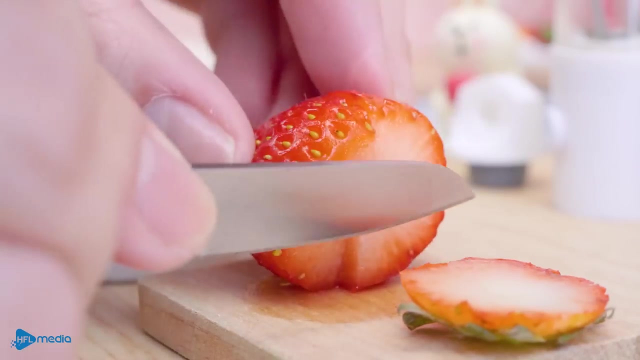 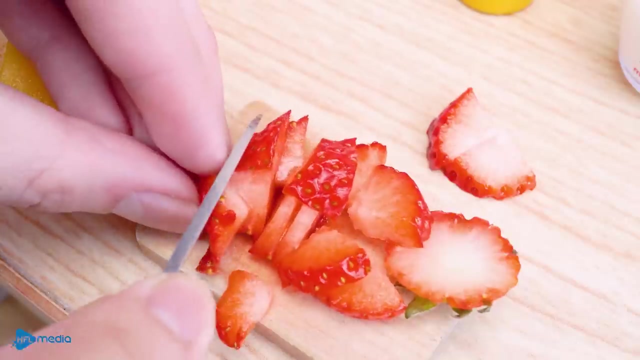 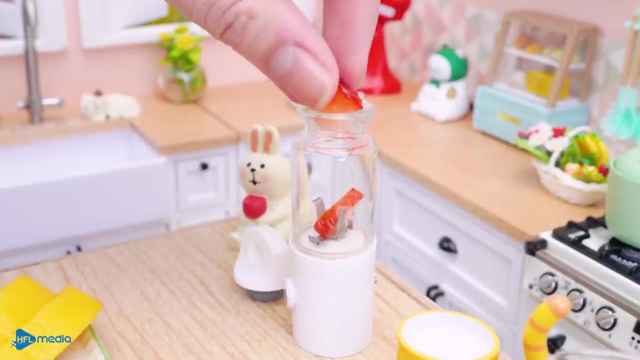 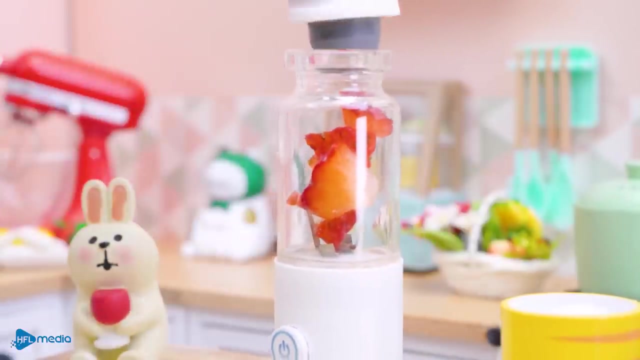 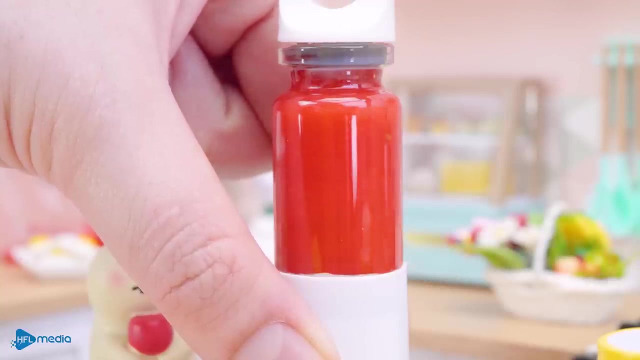 Thank you. I will make a rainbow lollipop. Cut the green onion into small pieces and put it in a blender to make the sauce. Add 1 tablespoon of soy sauce, 1 tablespoon of sugar and 1 tablespoon of cooking wine to the blender and blend. 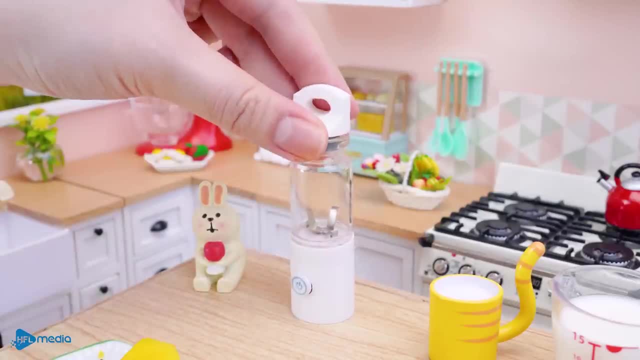 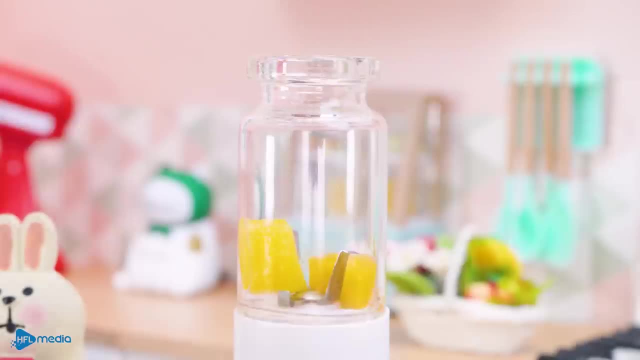 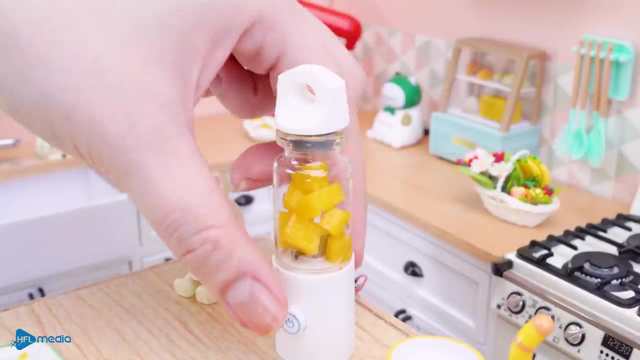 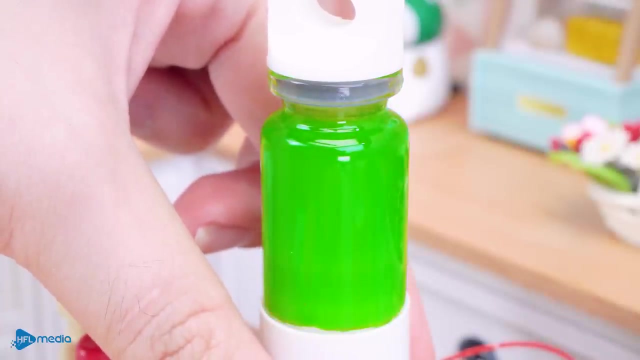 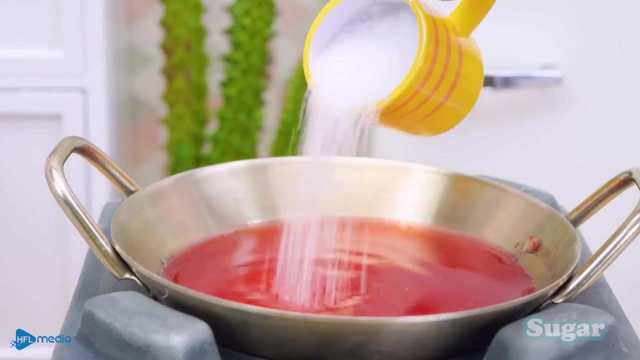 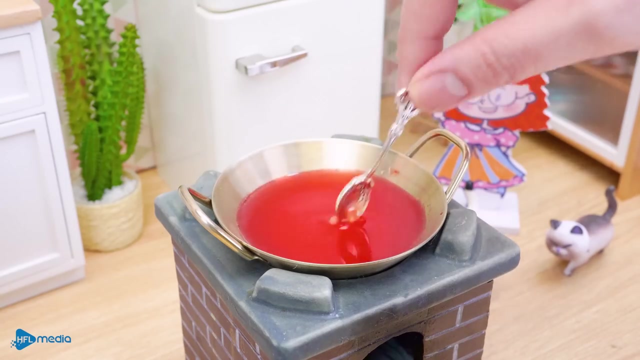 Add 1 tablespoon of fish sauce, 1 tablespoon of soy sauce, 2 tablespoons of cooking wine, 1 tablespoon of sugar to the blender and blend. Add 1 tablespoon of water. Add 1 tablespoon of cooking wine. Add a little water and mix. 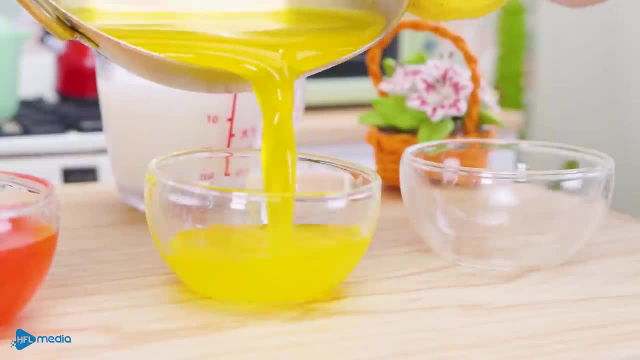 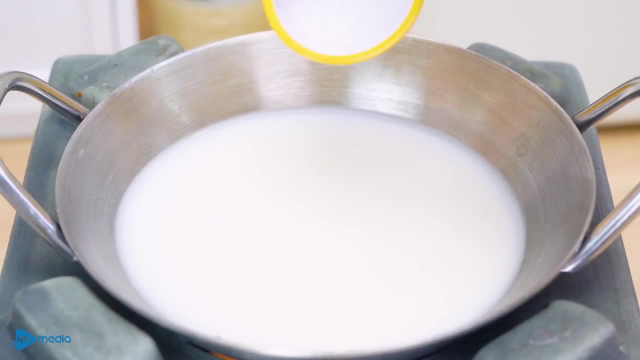 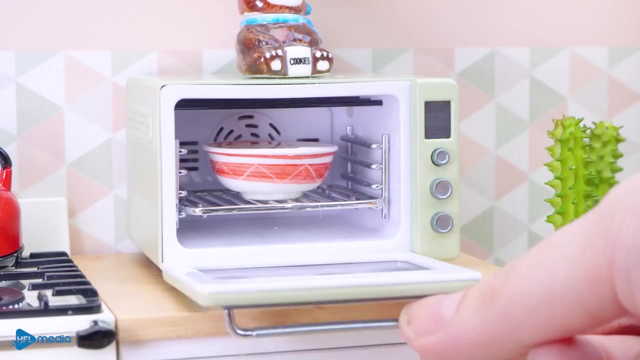 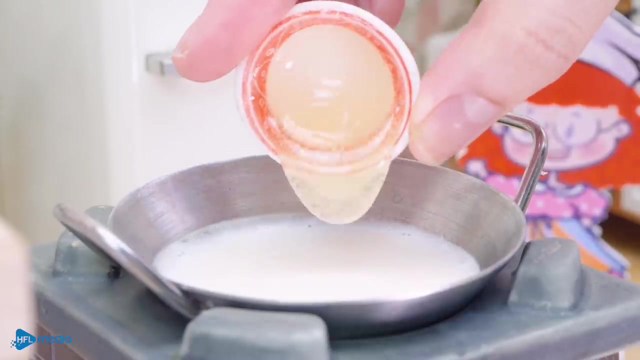 Add a little salt and mix. I'll make sweet and sour pork stew. I'll make sweet and sour pork stew. First, put a box of pork belly into a pot. Add a bit of salt and sugar. Whip the eggs well, Add some salt and sugar and mix with the eggs. 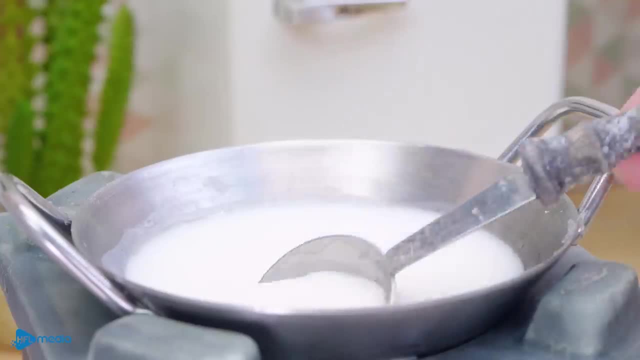 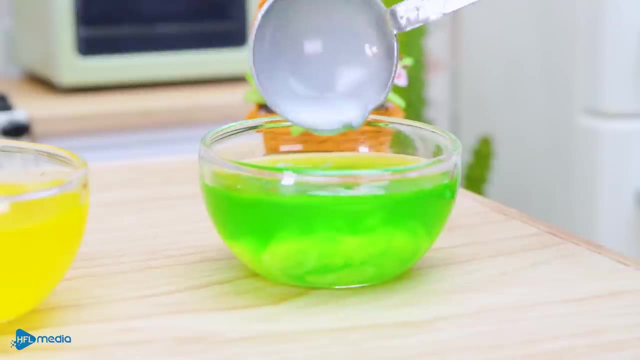 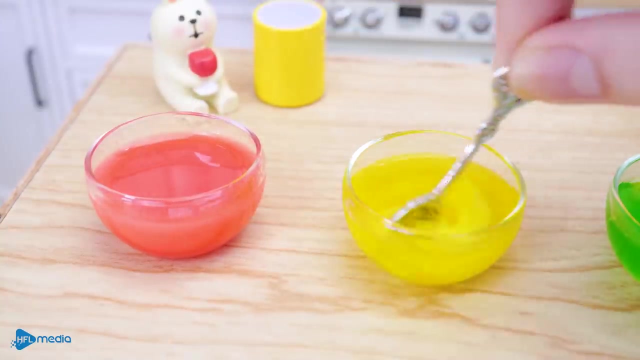 Add 1 the cooking wine, Add 1 the bread flour, Add 1.5 the egg yolk, Add 1.5 the water. Mix it well, 3. 2. 1. 1. 2.. 4. 3., 4. 3., 2., 2. 1.. 0.. 4. 2. 3. 1., 4. 2. 1. 1. 1.. 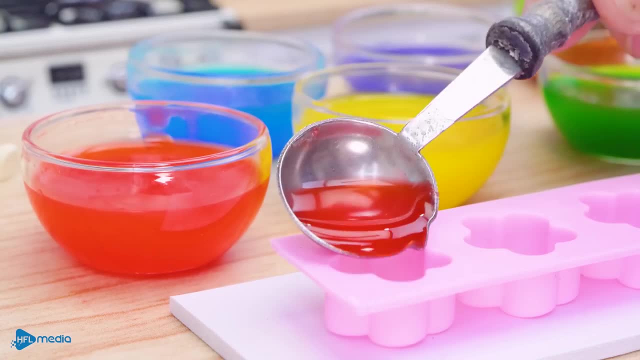 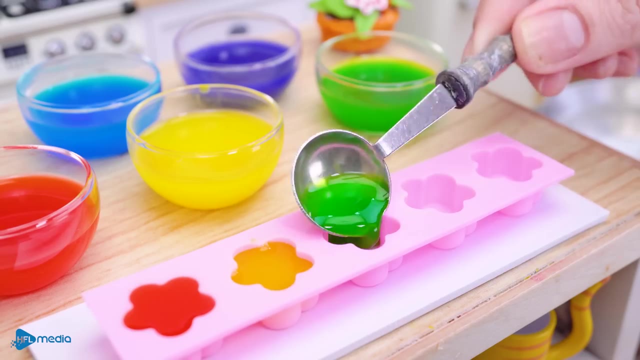 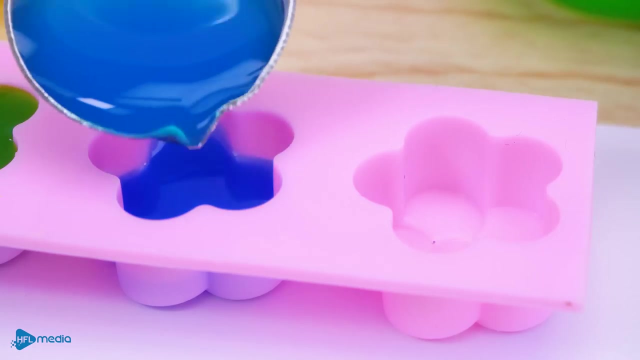 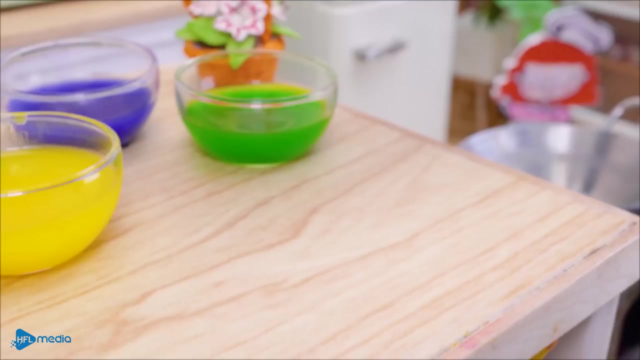 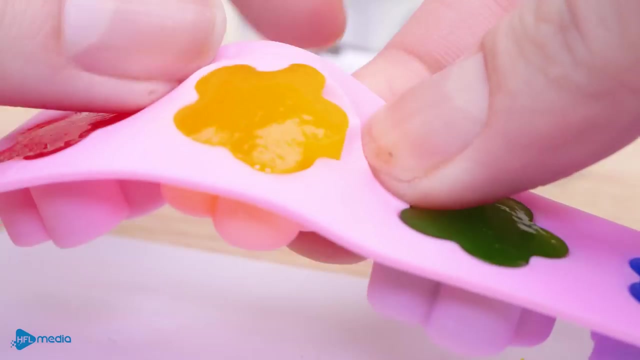 3., 2., 0., 2., 3., 5., 4.. Add 1 cup of water and 1 cup of soy sauce to the pot and boil it over high heat for 10 minutes. Add 1 cup of water and 1 cup of soy sauce to the pot and boil it for 10 minutes. 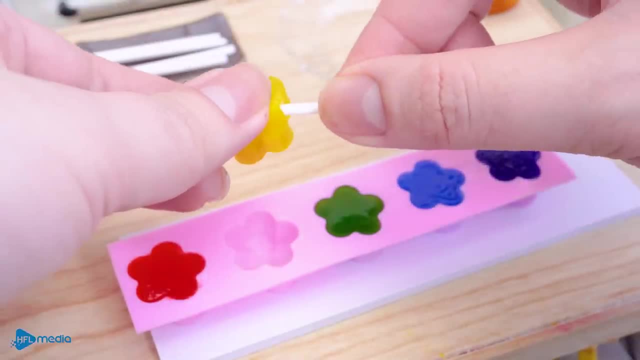 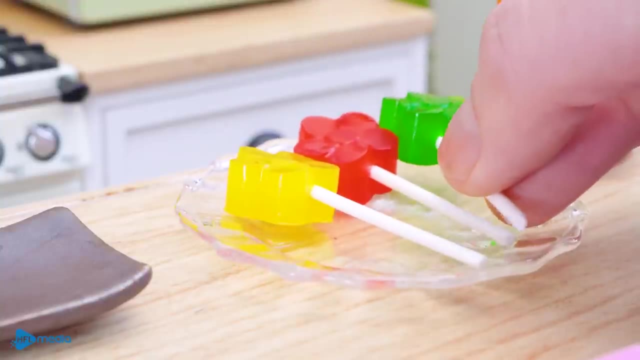 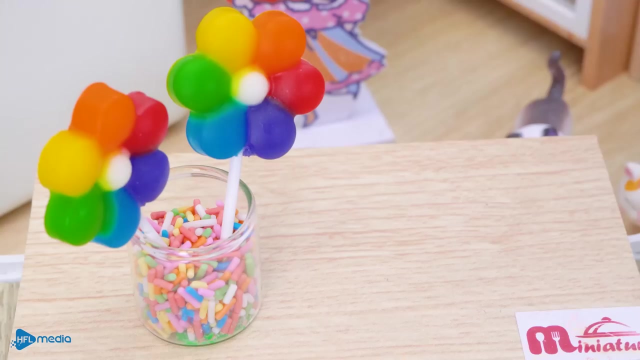 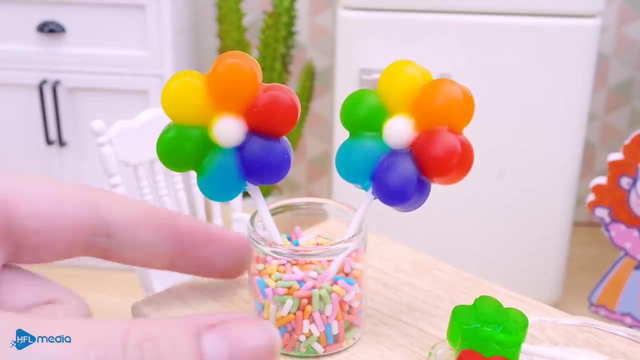 When the oil is enough, hotere's 10 fisheteens. Put it in a bowl. add 1 fooler, something white and a little bit ofíoil, and boil it. Add 2 cups of cold water. Let's taste it bro. 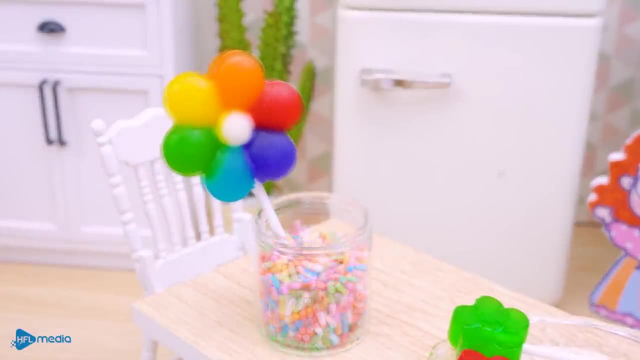 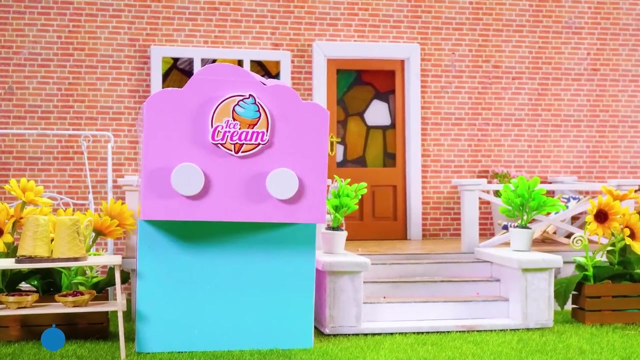 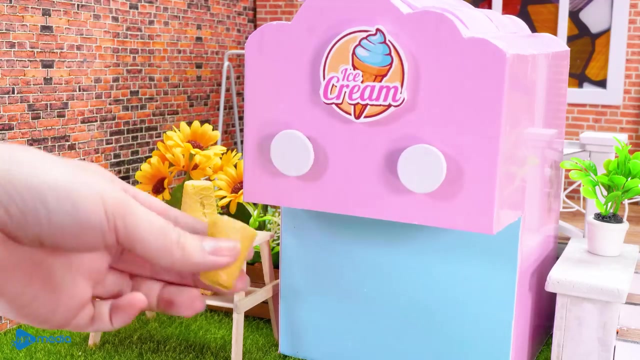 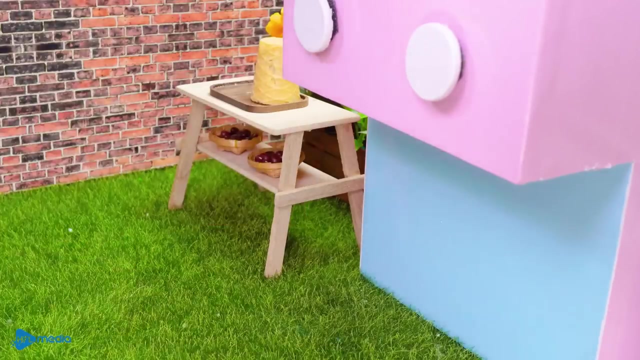 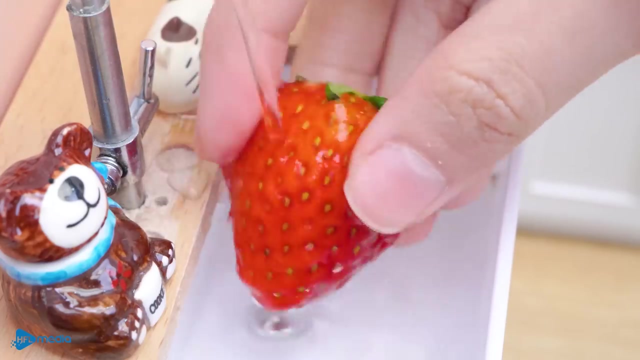 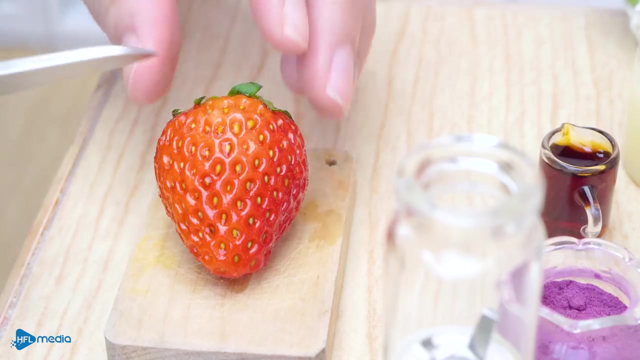 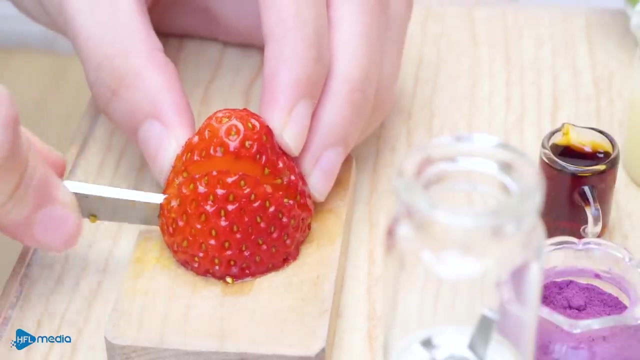 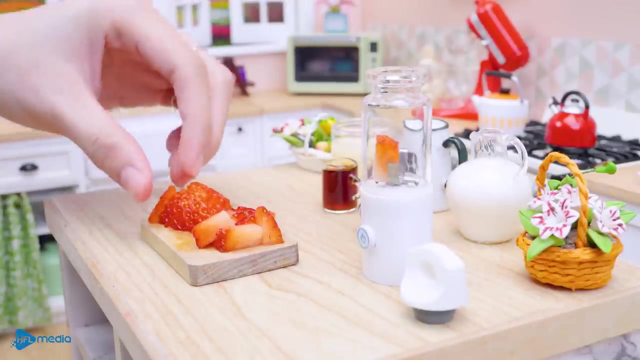 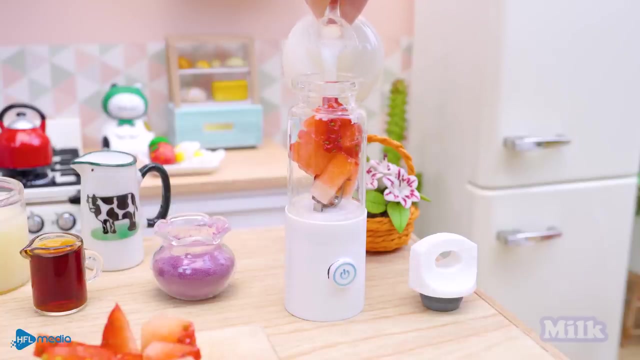 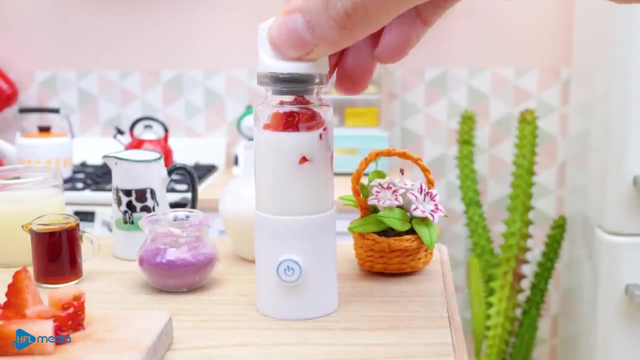 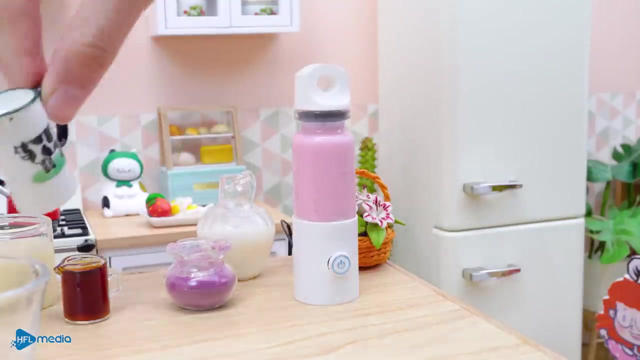 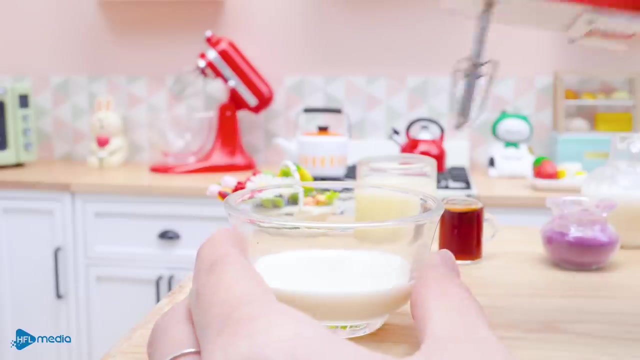 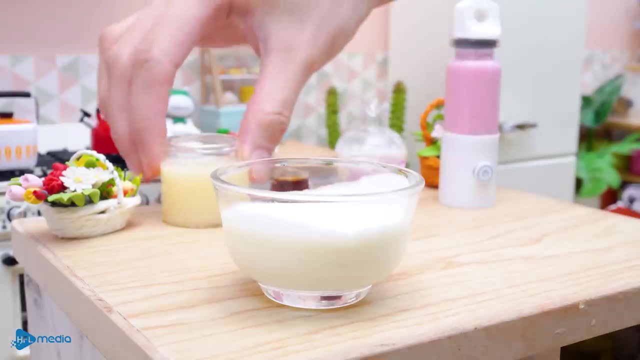 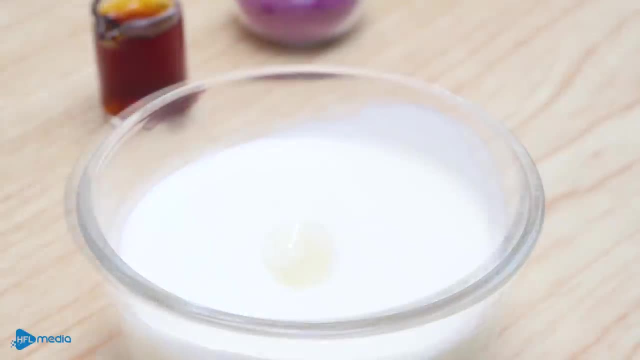 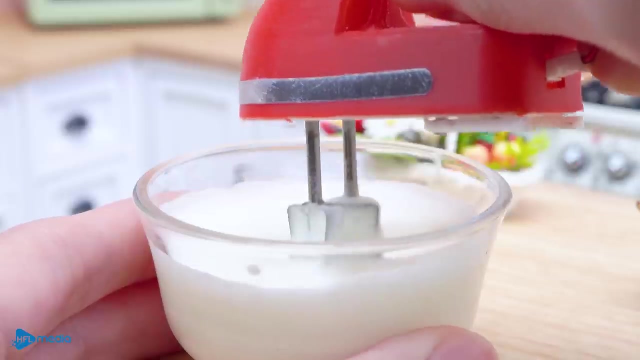 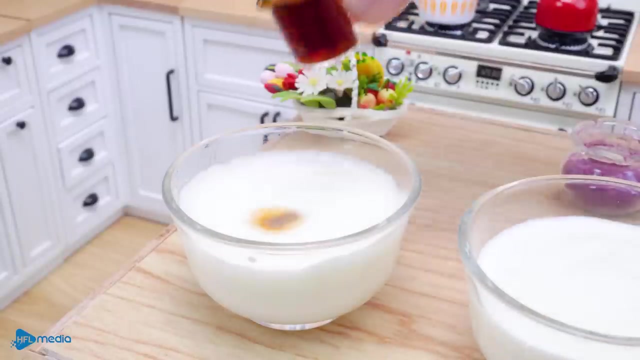 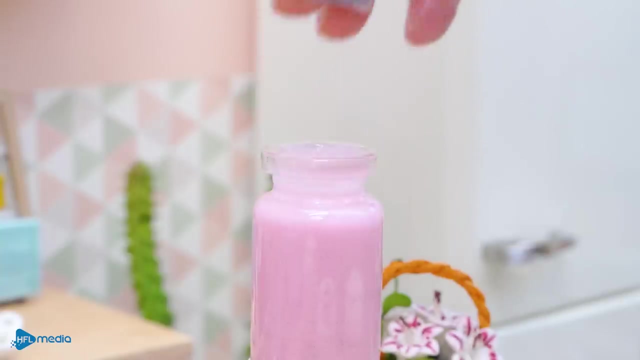 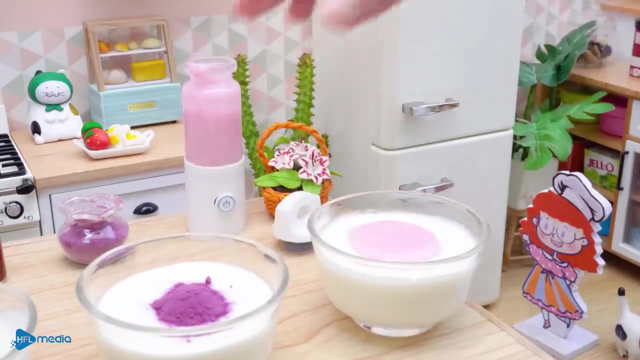 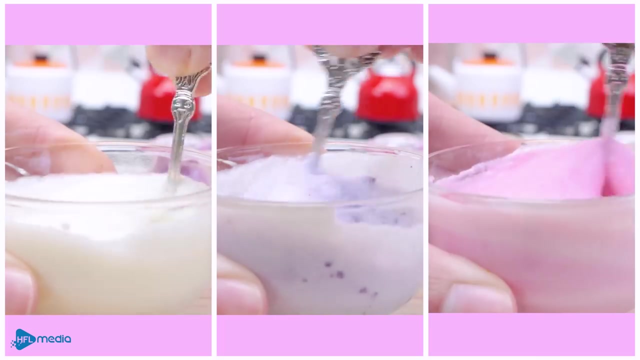 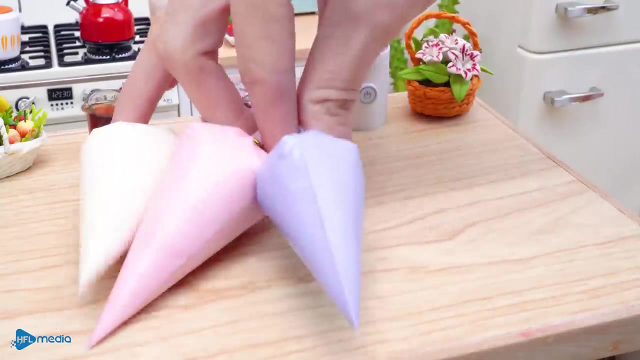 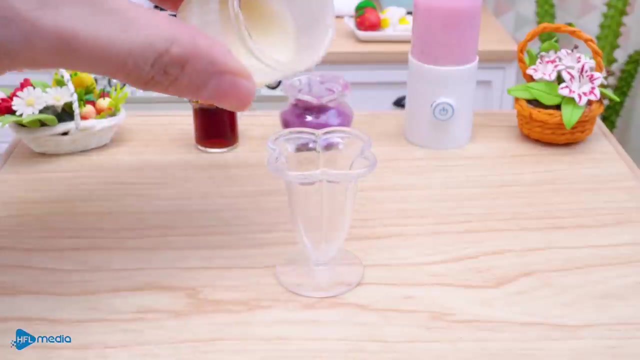 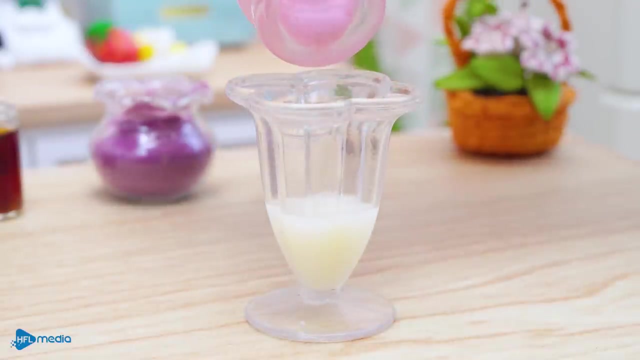 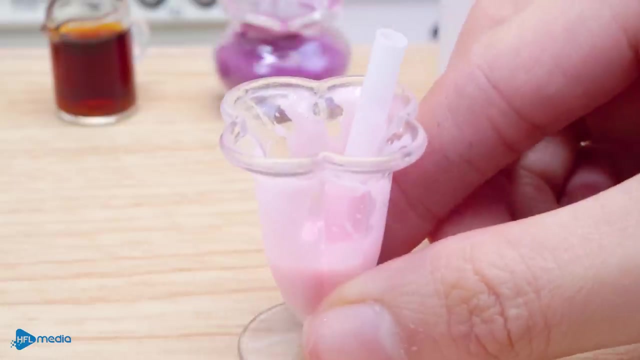 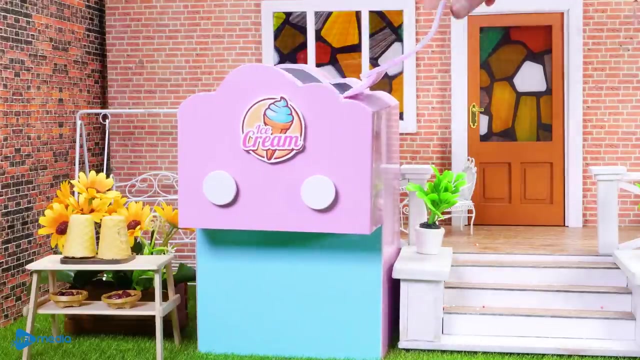 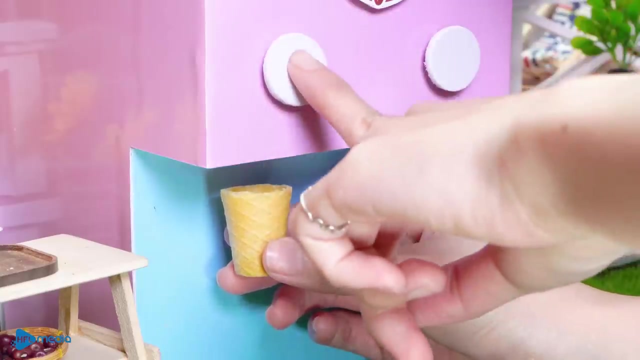 I have to rebuild the eye cream machine. I have to rebuild the eye cream machine. I have to rebuild the eye cream machine Blurrrrrrrrrrrrrrrrrrrrrrrrrrrrrrrrrrrrrrrrrrrrrrrrrrrrrrrrrrrrrrrrrrrrrrrrrrrrrrrrrrrrrrrrrrrrrrrrrrrrrrrrrrrrrrrrrrrrrrrrrrrrrrrrrrrrrrrrrrrrrrrrrrrrrrrrrrrrrrrrrrrrrrrrrrrrrrrrrrrrrrrrrrrrrrrrrrrrrrrrrrrrrrrrrrrrrrrrrrrrrrrrrrrrrrrrrrrrrrrrrrrrrrrrrrrrrrrrrrrrrrrrrrrrrrrrrrrrrrrrrrrrrrrrrrrrrrrrrrrrrrrrrrrrrrrrrrrrrrrrrrrrrrrrrrrrrrrrrrrrrrrrrrrrrrrrrrrrrrrrrrrrrrrrrrrrrrrrrrrrrrrrrrrrrrrrrrrrrrrrrrrrrrrrrrrrrrrrrrrrrrrrrrrrrrrrrrrrrrrrrrr. 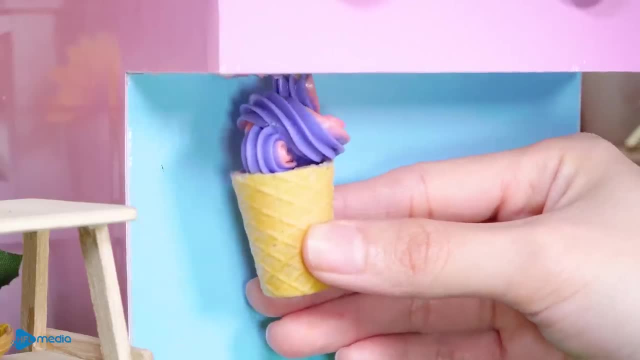 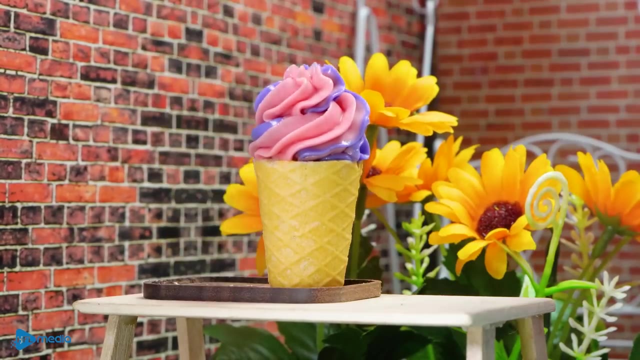 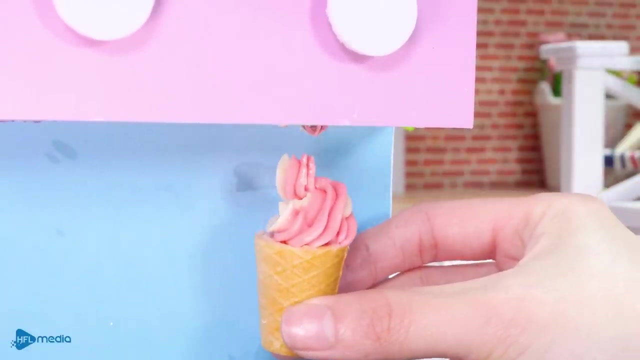 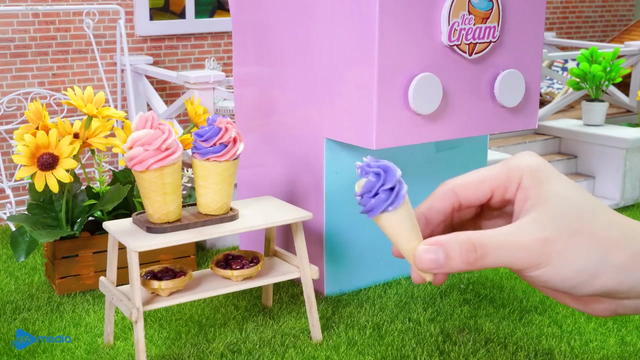 rrrrrrrrrrrrrrrrrrrrrrrrrrrrrrrrrrrrrrrrrrrrrrrrrrrrrrrrrrrrrrrrrrrrrrrrrrrrrrrrrrrrrrrrrrrrrrrrrrrrrrrrrrrrrrrrrrrrrrrrrrrrrrrrrrrrrrrrrrrrrrrrrrrrrrrrrrrrrrrrrrrrrrrrrrrrrrrrrrrrrrrrrrrrrrrrrrrrrrrrrrrrrrrrrrrrrrrrrrrrrrrrrrrrrrrrrrrrrrrrrrrrrrrrrrrrrrrrrrrrrrrrrrrrrrrrrrrrrrrrrrrrrrrrrrrrrrrrrrrrrrrrrrrrrrrrrrrrrrrrrrrrrrrrrrrrrrrrrrrrrrrrrrrrrrrrrrrrrrrrrrrrrrrrrrrrrrrrrrrrrrrrrrrrrrrrrrrrrrrrrrrrrrrrrrrrrrrrrrrrrrrrrrrrrrrrrrrrrrrrr. 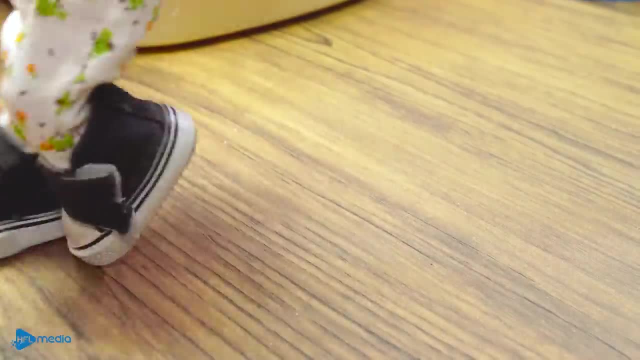 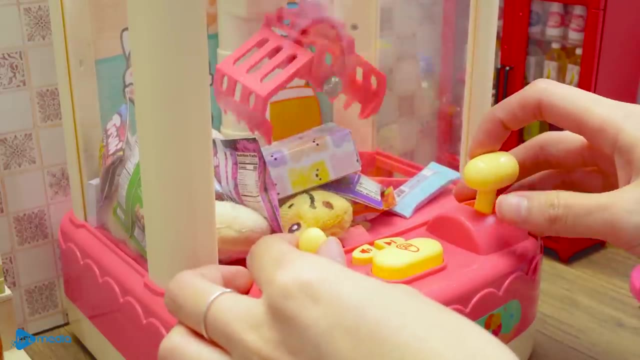 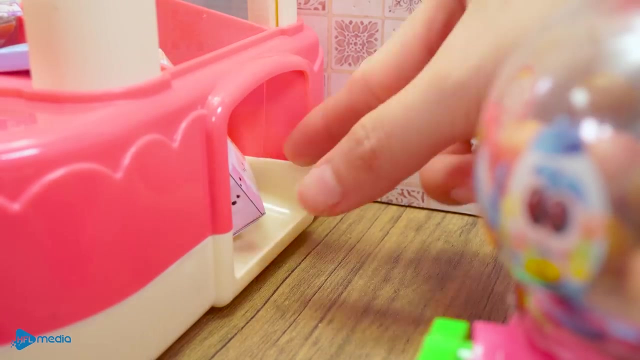 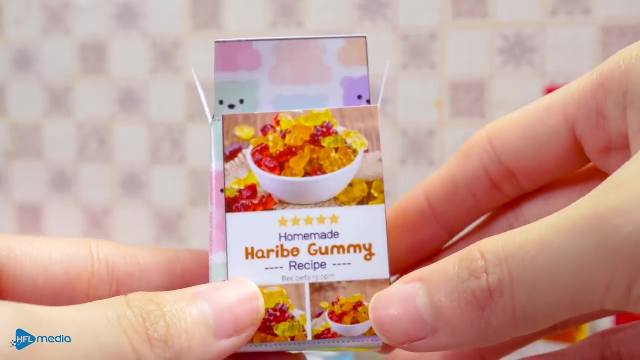 rrrrrrrrrrrrrrrrrrrrrrrrrrrrrrrrrrrrrrrrrrrrrrrrrrrrrrrrrrrrrrrrrrrrrrrrrrrrrrrrrrrrrrrrrrrrrrrrrrrrrrrrrrrrrrrrrrrrrrrrrrrrrrrrrrrrrrrrrrrrrrrrrrrrrrrrrrrrrrrrrrrrrrrrrrrrrrrrrrrrrrrrrrrrrrrrrrrrrrrrrrrrrrrrrrrrrrrrrrrrrrrrrrrrrrrrrrrrrrrrrrrrrrrrrrrrrrrrrrrrrrrrrrrrrrrrrrrrrrrrrrrrrrrrrrrrrrrrrrrrrrrrrrrrrrrrrrrrrrrrrrrrrrrrrrrrrrrrrrrrrrrrrrrrrrrrrrrrrrrrrrrrrrrrrrrrrrrrrrrrrrrrrrrrrrrrrrrrrrrrrrrrrrrrrrrrrrrrrrrrrrrrrrrrrrrrrrrrrrrrr. 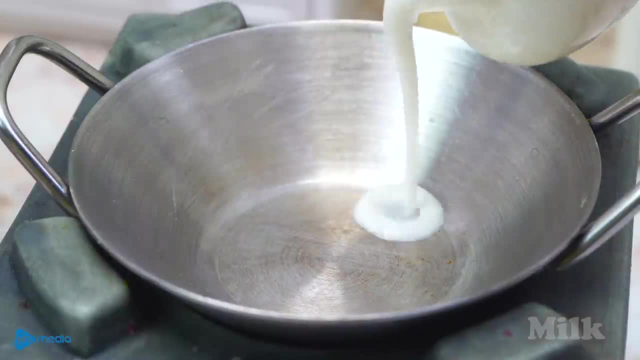 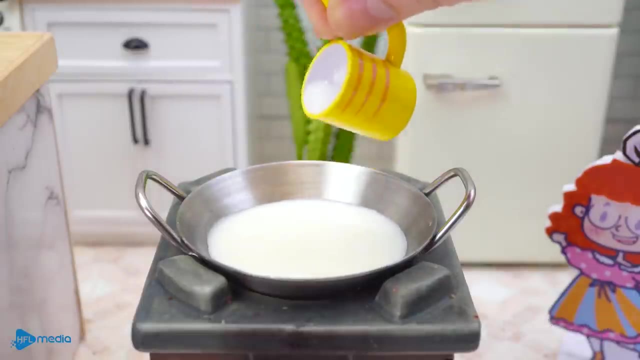 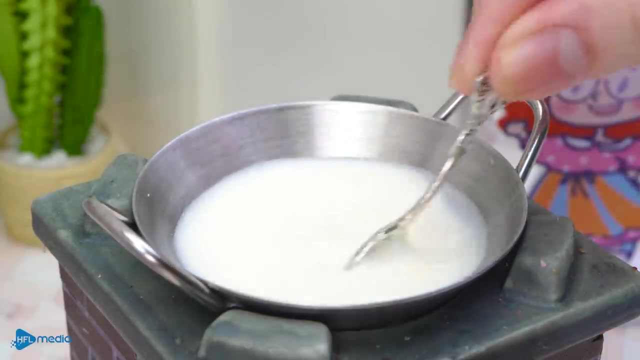 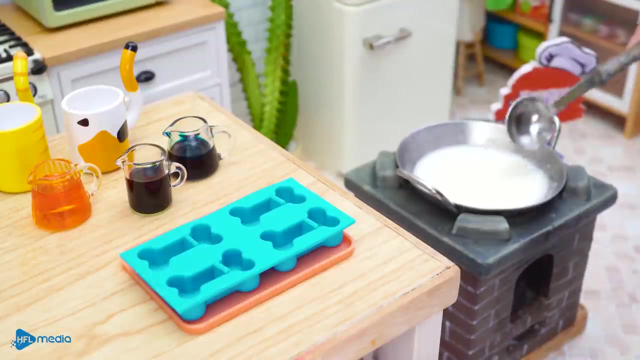 rrrrrrrrrrrrrrrrrrrrrrrrrrrrrrrrrrrrrrrrrrrrrrrrrrrrrrrrrrrrrrrrrrrrrrrrrrrrrrrrrrrrrrrrrrrrrrrrrrrrrrrrrrrrrrrrrrrrrrrrrrrrrrrrrrrrrrrrrrrrrrrrrrrrrrrrrrrrrrrrrrrrrrrrrrrrrrrrrrrrrrrrrrrrrrrrrrrrrrrrrrrrrrrrrrrrrrrrrrrrrrrrrrrrrrrrrrrrrrrrrrrrrrrrrrrrrrrrrrrrrrrrrrrrrrrrrrrrrrrrrrrrrrrrrrrrrrrrrrrrrrrrrrrrrrrrrrrrrrrrrrrrrrrrrrrrrrrrrrrrrrrrrrrrrrrrrrrrrrrrrrrrrrrrrrrrrrrrrrrrrrrrrrrrrrrrrrrrrrrrrrrrrrrrrrrrrrrrrrrrrrrrrrrrrrrrrrrrrrrrr. 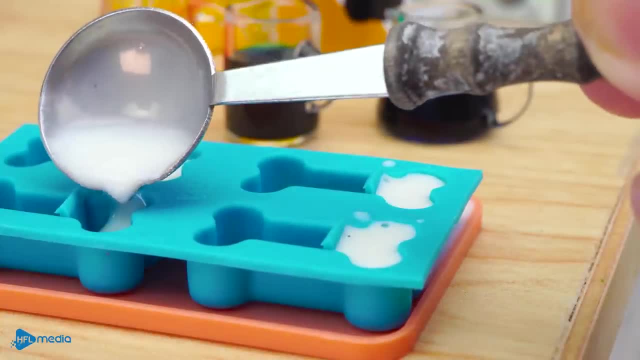 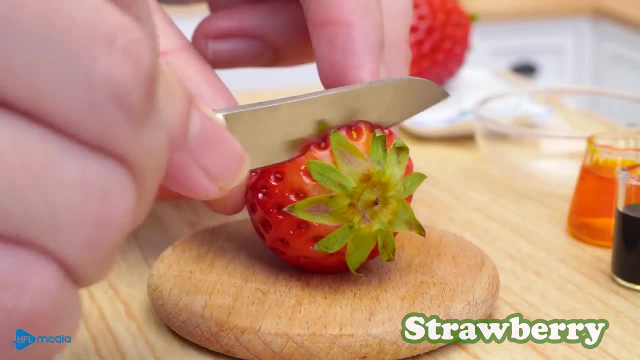 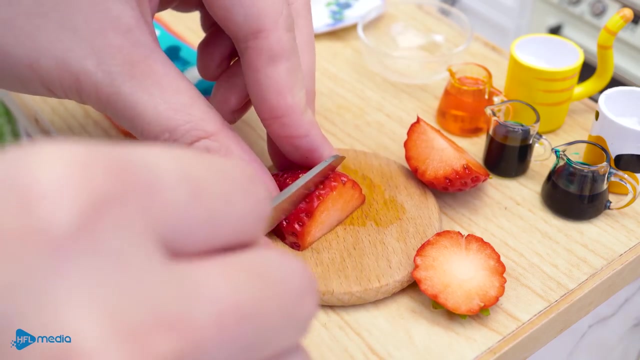 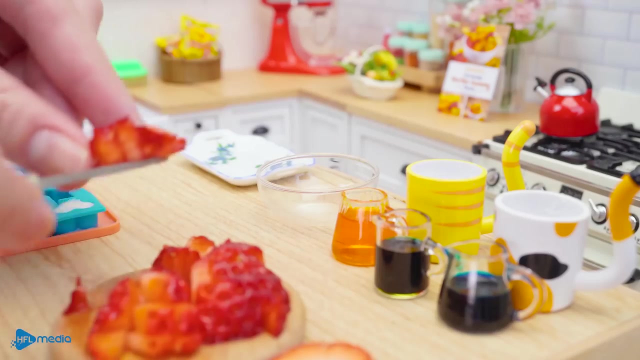 rrrrrrrrrrrrrrrrrrrrrrrrrrrrrrrrrrrrrrrrrrrrrrrrrrrrrrrrrrrrrrrrrrrrrrrrrrrrrrrrrrrrrrrrrrrrrrrrrrrrrrrrrrrrrrrrrrrrrrrrrrrrrrrrrrrrrrrrrrrrrrrrrrrrrrrrrrrrrrrrrrrrrrrrrrrrrrrrrrrrrrrrrrrrrrrrrrrrrrrrrrrrrrrrrrrrrrrrrrrrrrrrrrrrrrrrrrrrrrrrrrrrrrrrrrrrrrrrrrrrrrrrrrrrrrrrrrrrrrrrrrrrrrrrrrrrrrrrrrrrrrrrrrrrrrrrrrrrrrrrrrrrrrrrrrrrrrrrrrrrrrrrrrrrrrrrrrrrrrrrrrrrrrrrrrrrrrrrrrrrrrrrrrrrrrrrrrrrrrrrrrrrrrrrrrrrrrrrrrrrrrrrrrrrrrrrrrrrrrrrr. 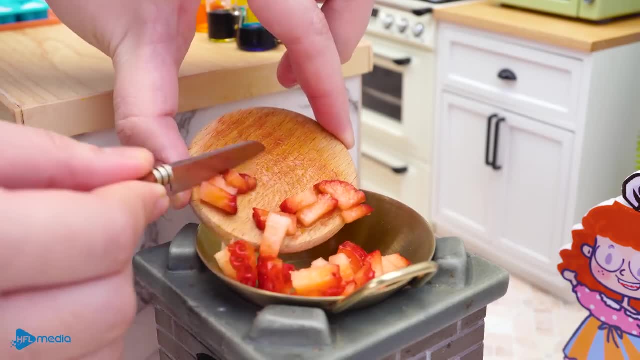 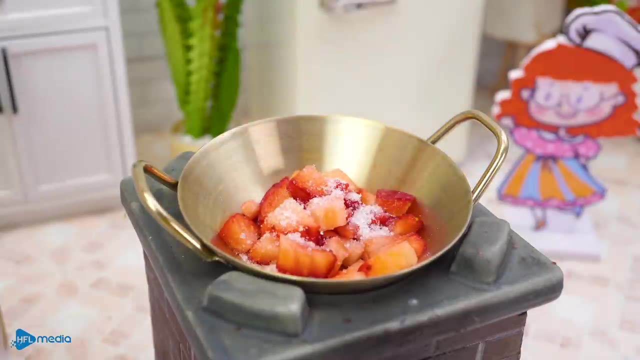 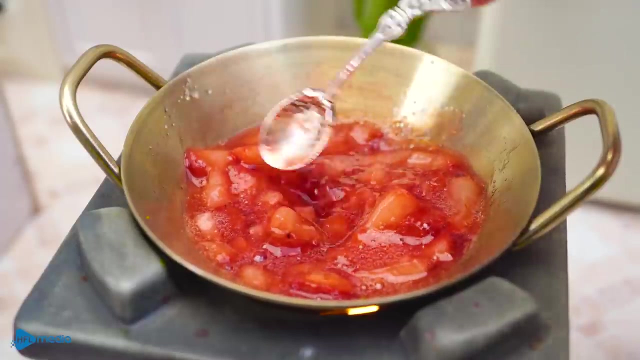 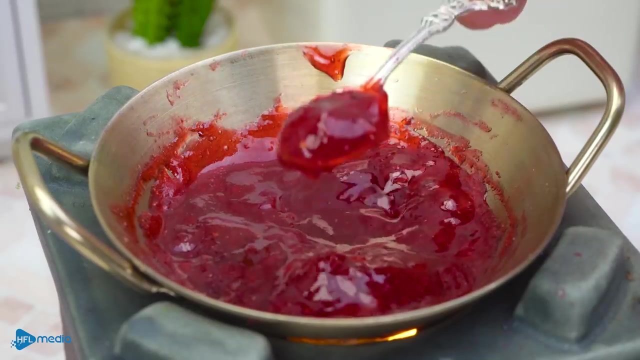 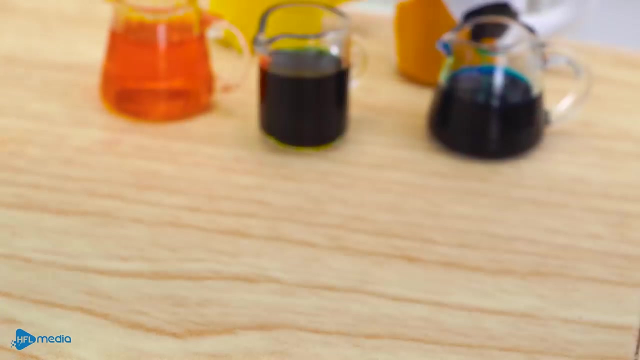 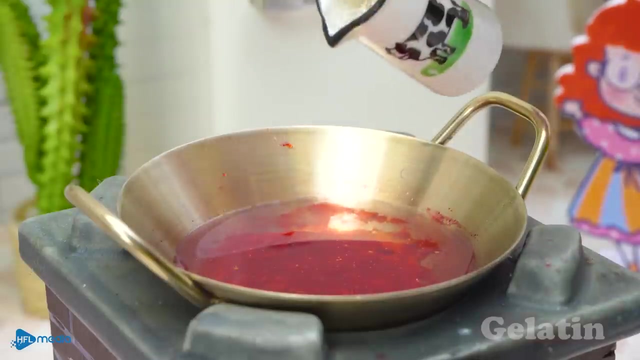 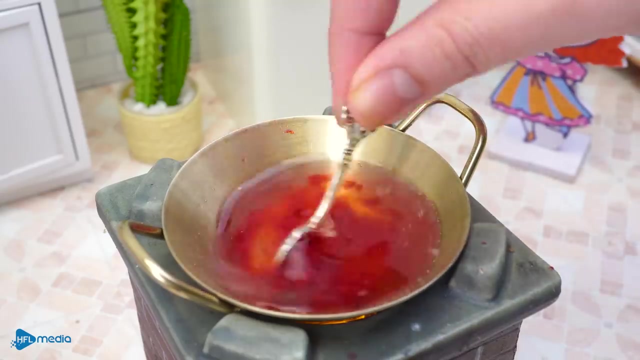 You can definitely make it at home. You can get something to drink hiking in Korea. Add the jjajang sauce and the spicy sauce. Add the jjajang sauce. Add the jjajang sauce. Mix them well. Pour the hot water in a pot. 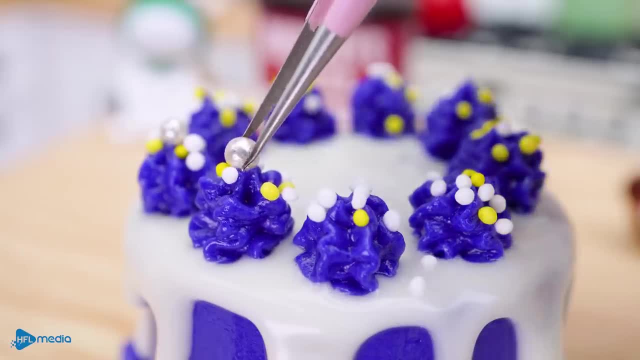 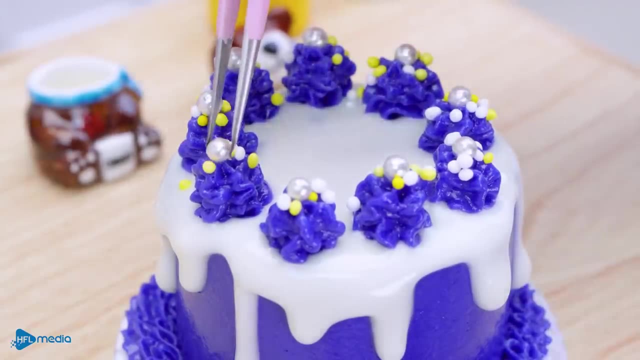 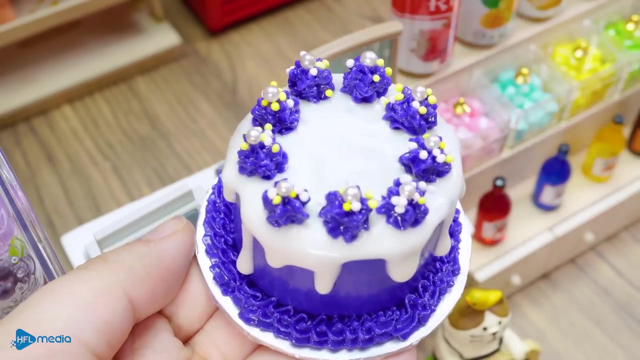 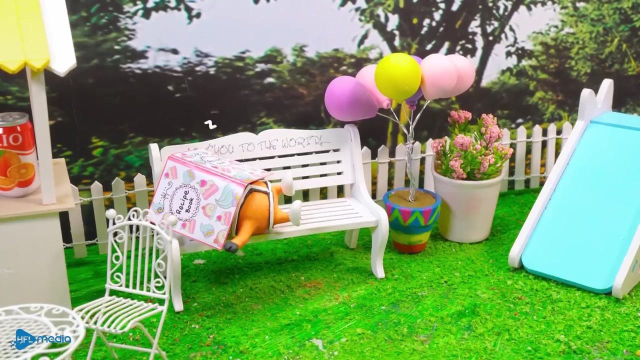 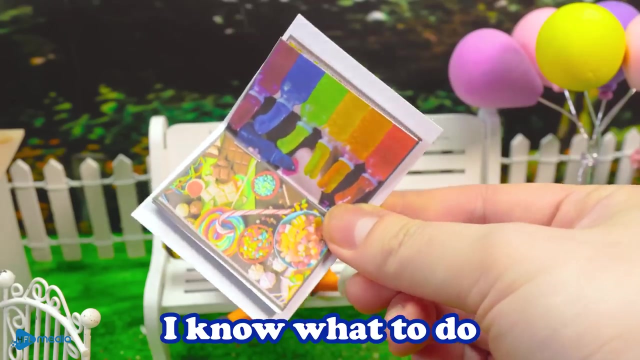 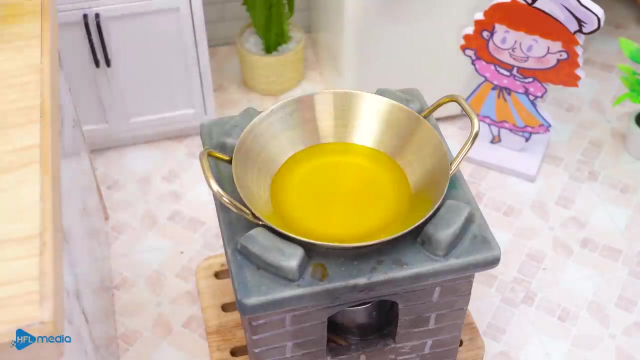 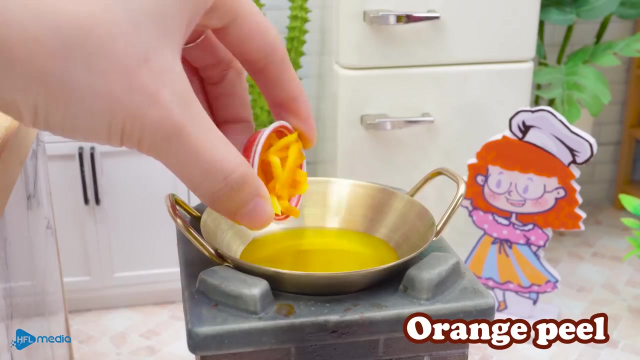 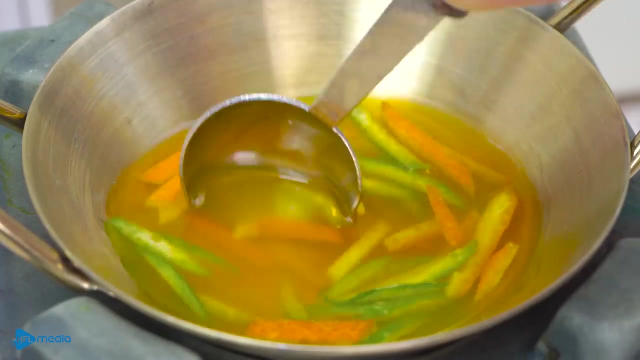 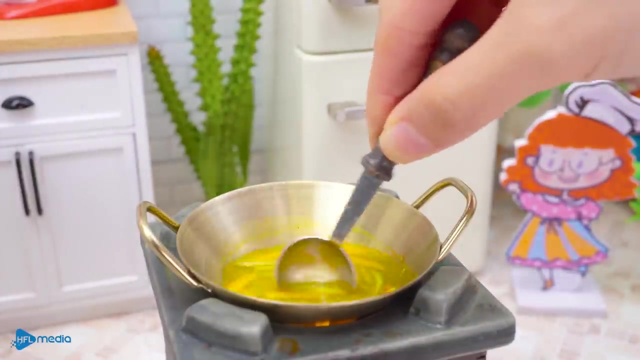 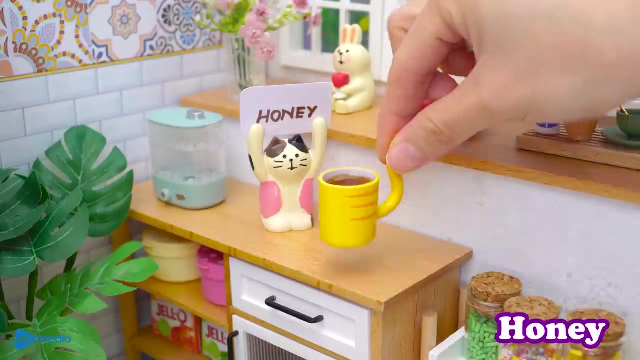 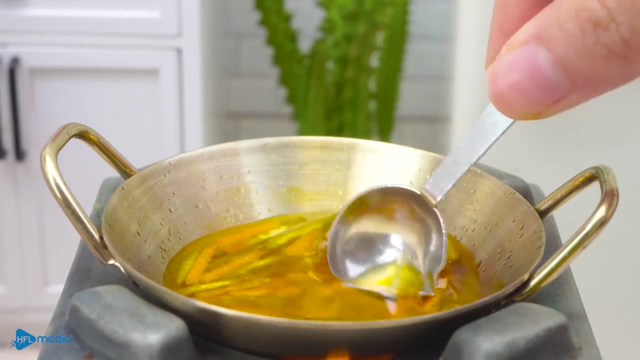 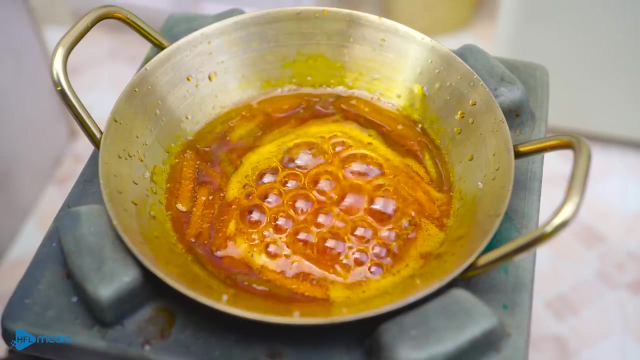 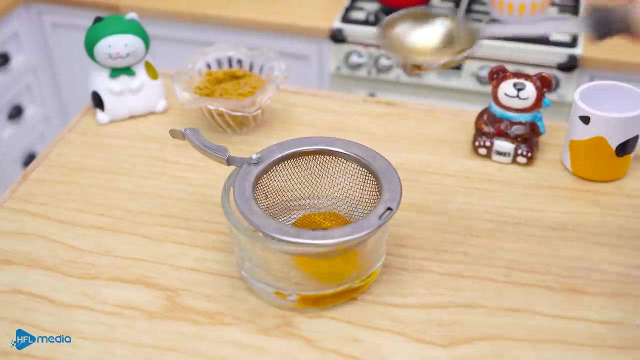 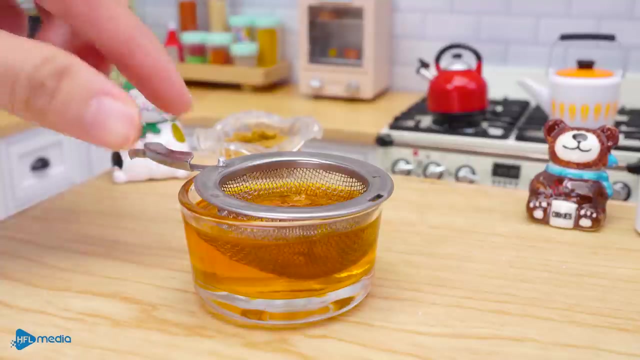 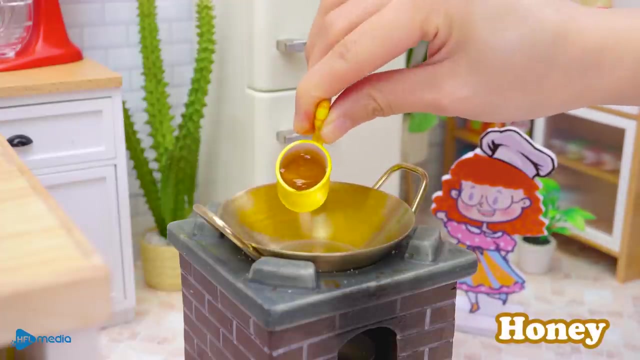 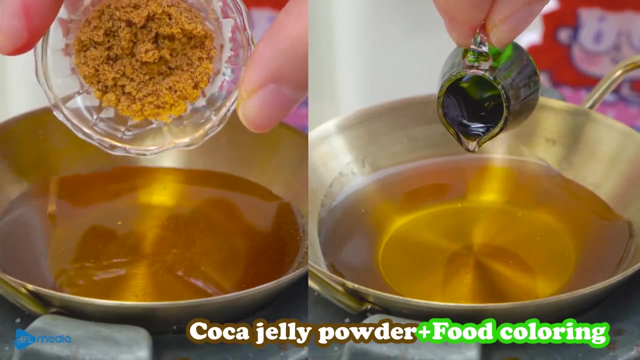 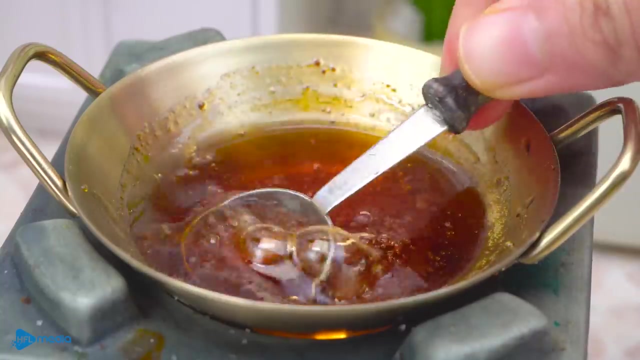 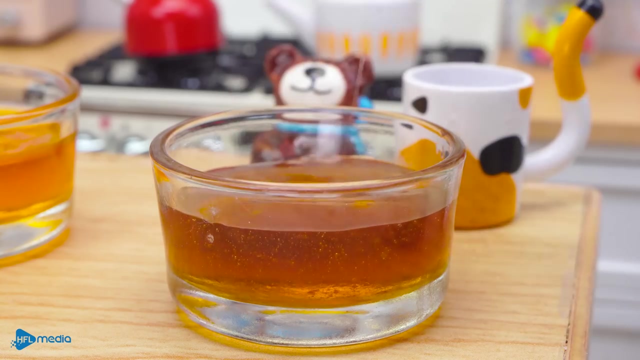 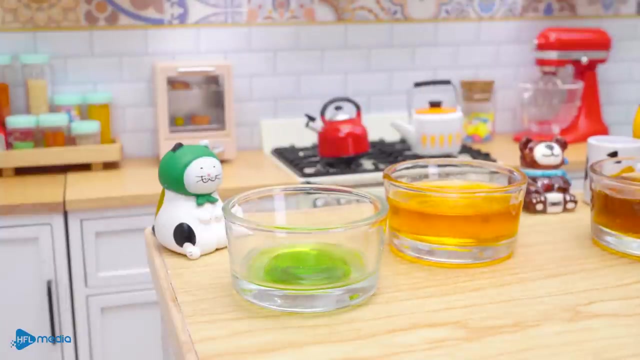 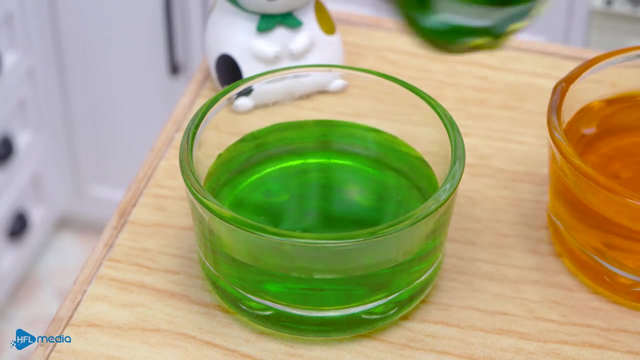 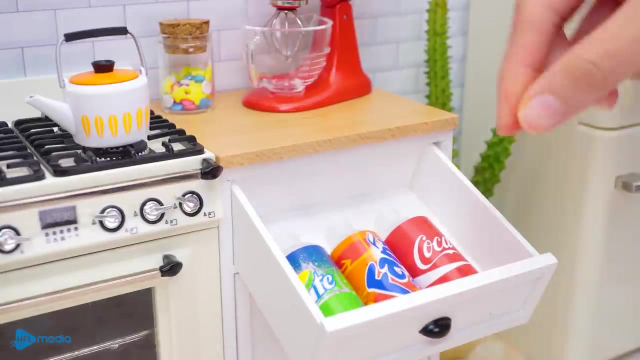 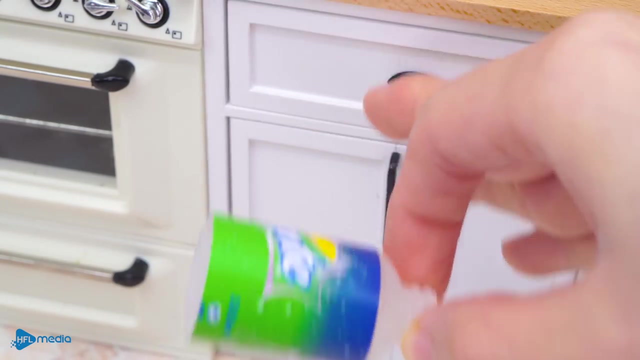 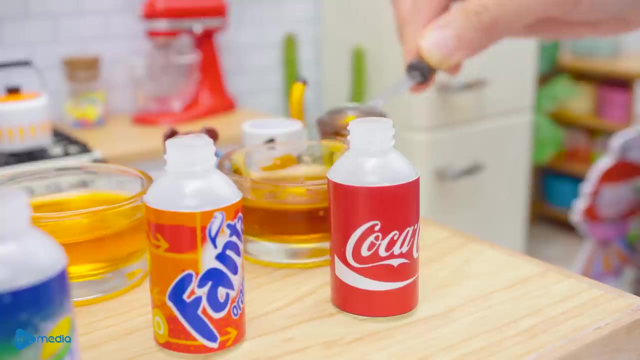 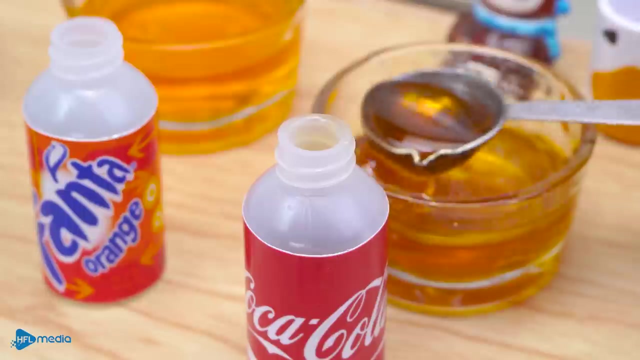 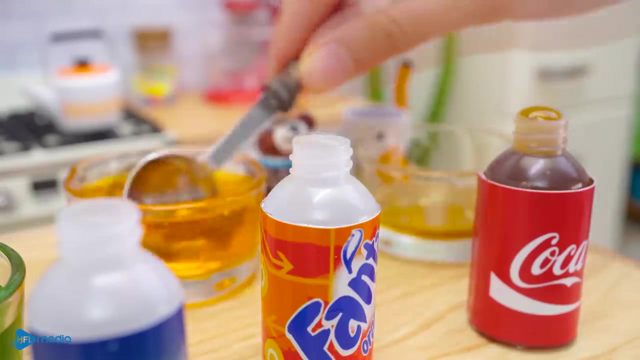 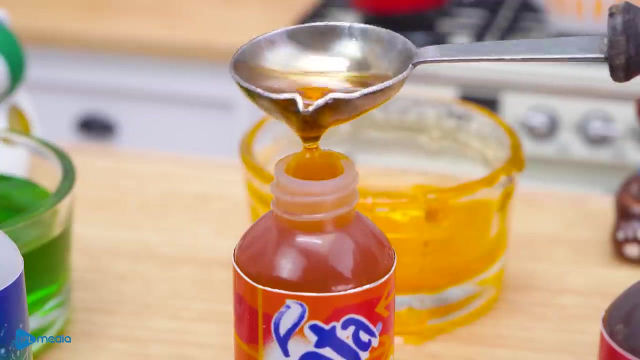 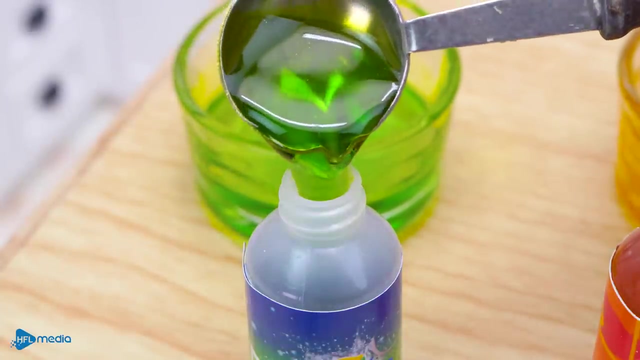 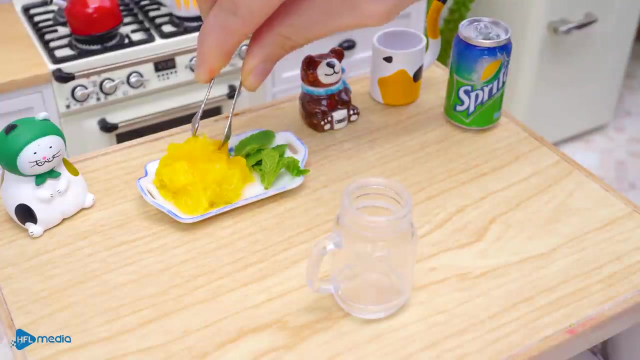 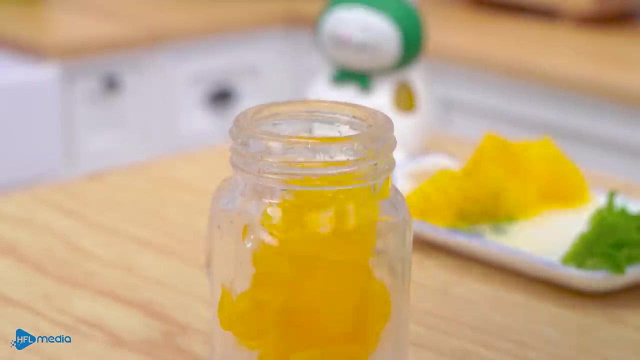 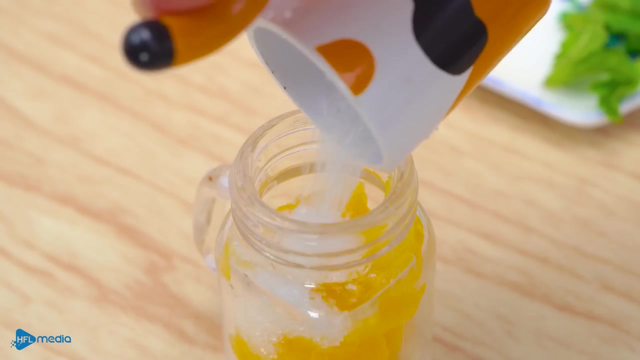 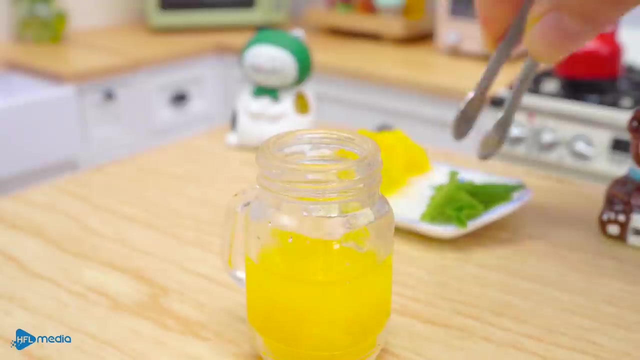 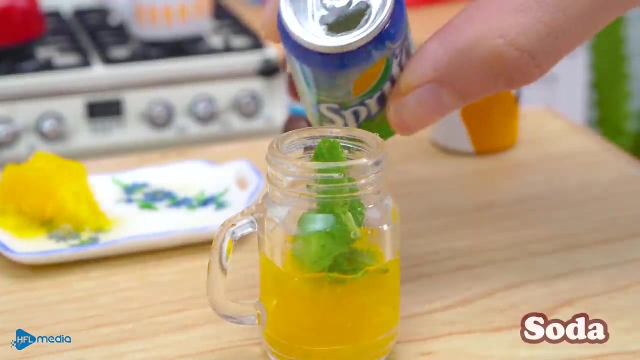 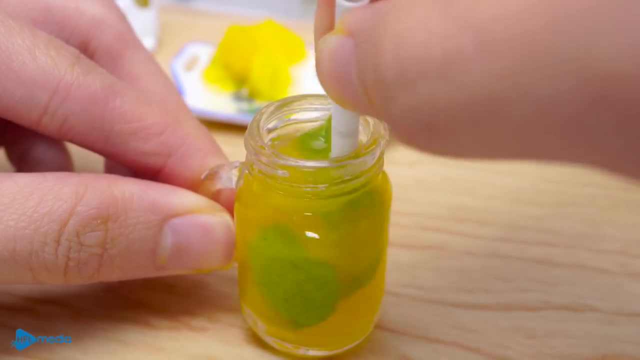 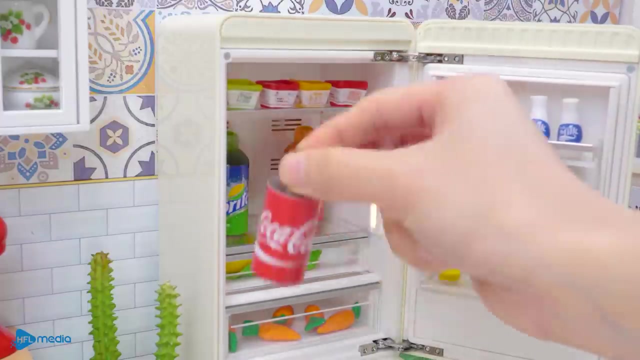 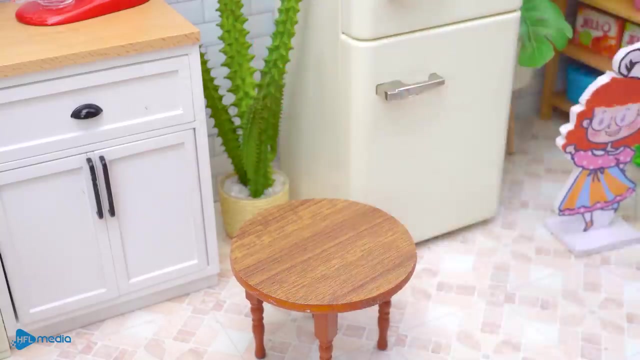 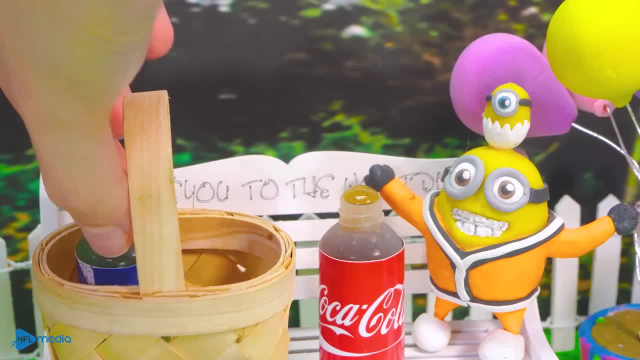 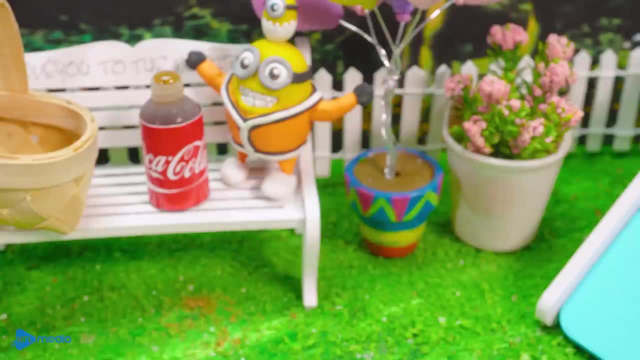 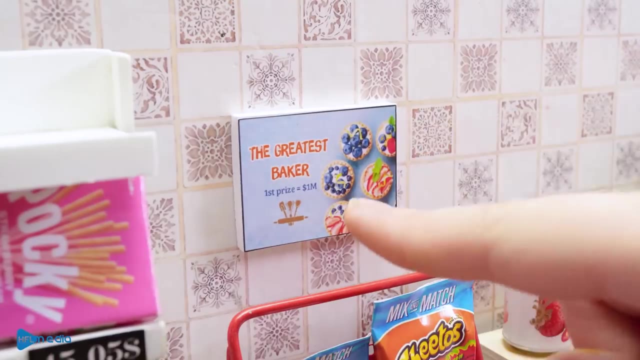 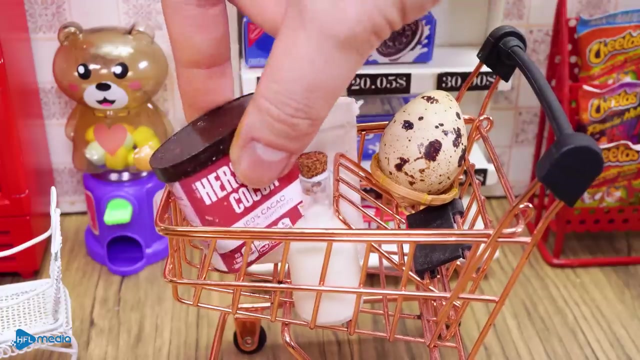 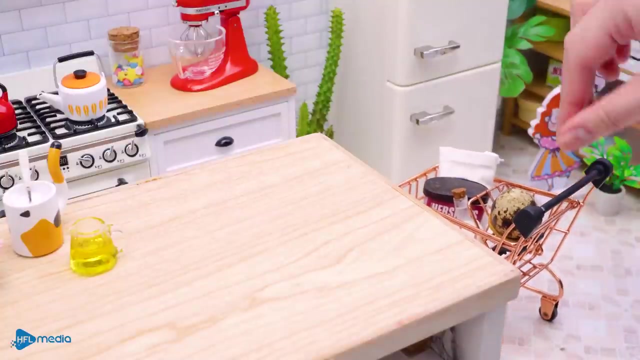 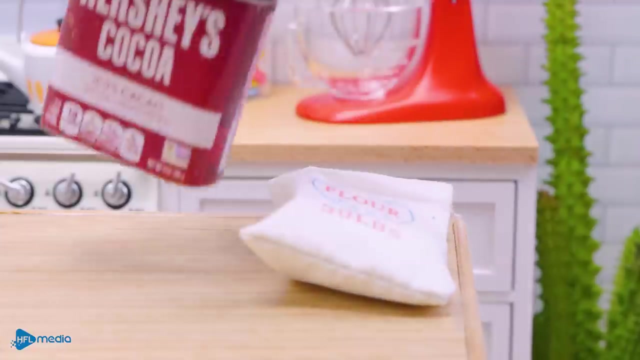 Here you are. Wow, delectable, Wow, I will be the champion. Aha, Put a lot of ingredients in the food processor and mix well. Add a little bit of cooking oil and mix well. Put the pork belly in a bowl. 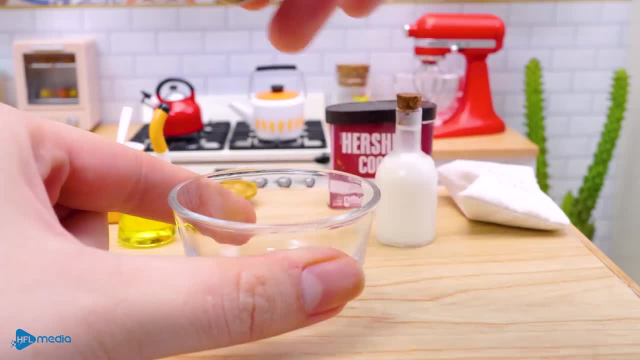 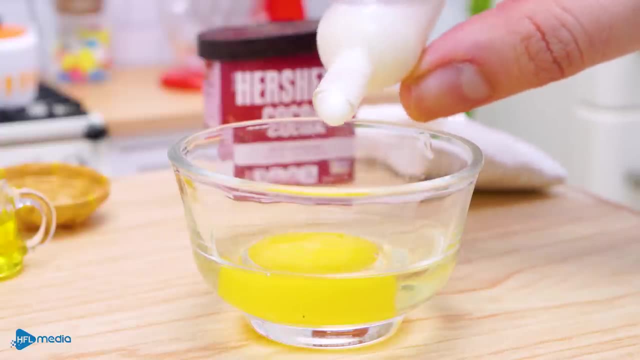 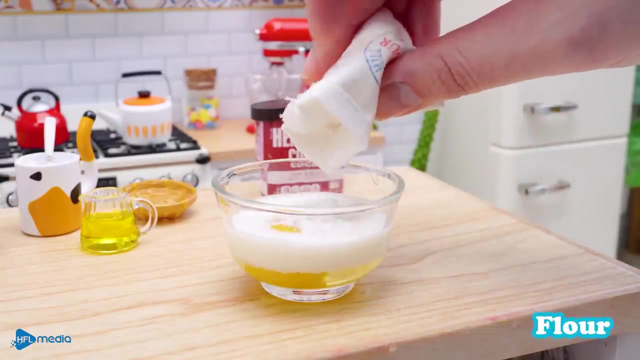 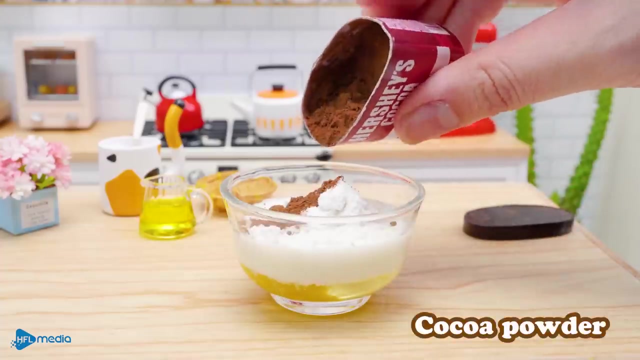 Put the pork belly in a bowl and mix well. Add a little bit of salt and pepper. Pour the milk into the pot. Add the sugar, Mix well. Add the egg. Add the sugar, Mix well. Add the egg. Add the salt. 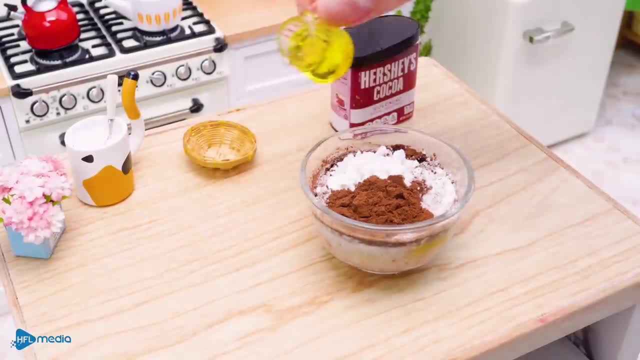 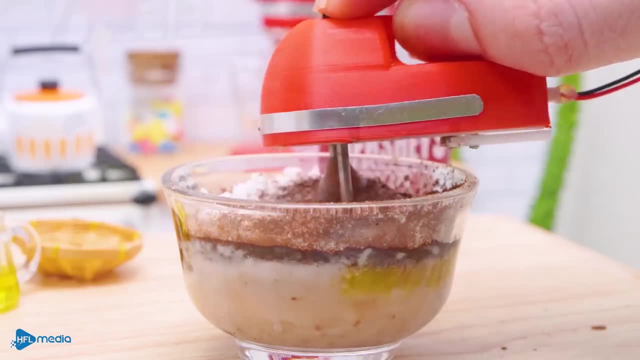 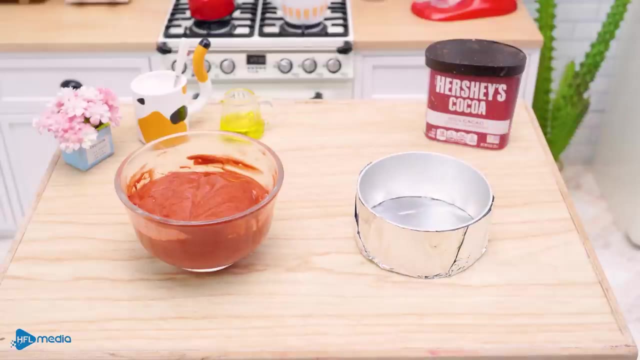 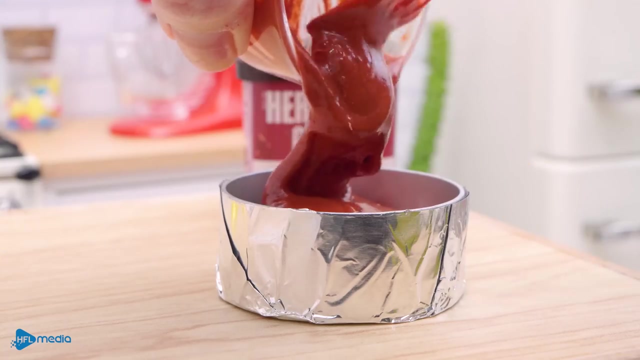 Add the pepper. Add the garlic, Add the soy sauce. Mix well, 會 piping bag. The dough-shaped dough preheats 45°C in 5 minutes. Add milk on a boiling pan. Add 2 eggs. Add milk on a hot pan. 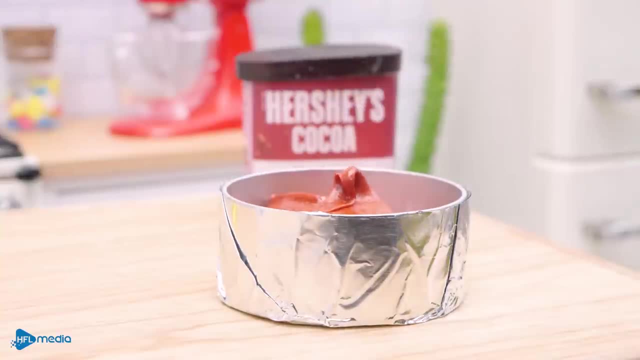 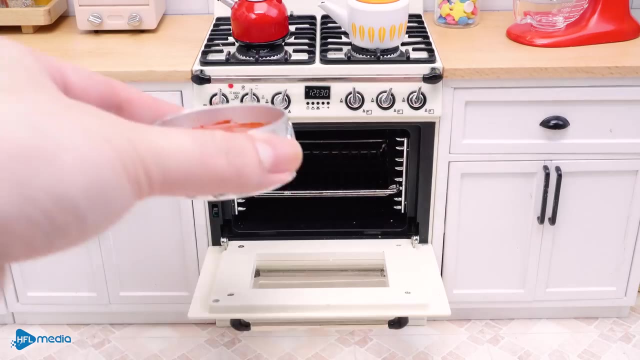 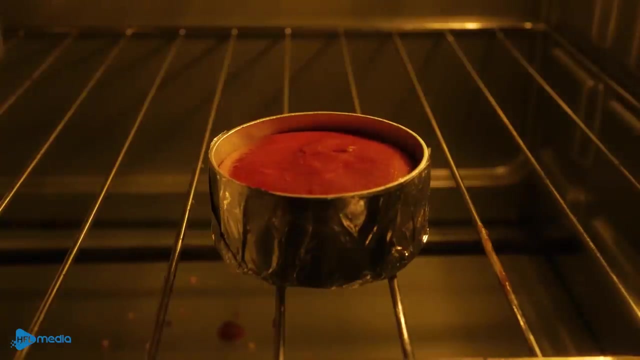 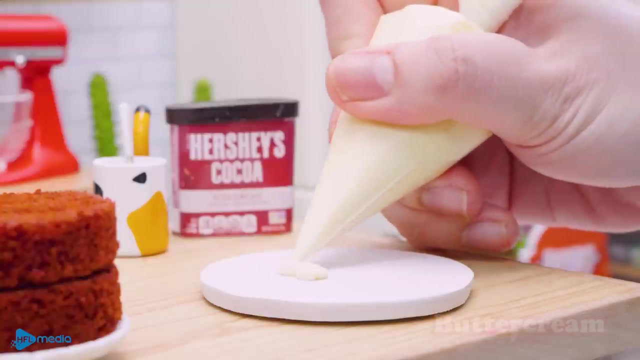 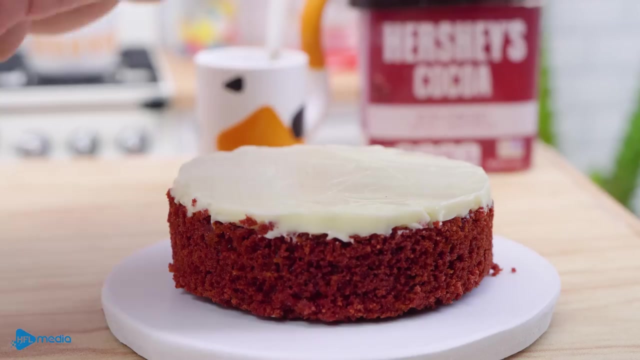 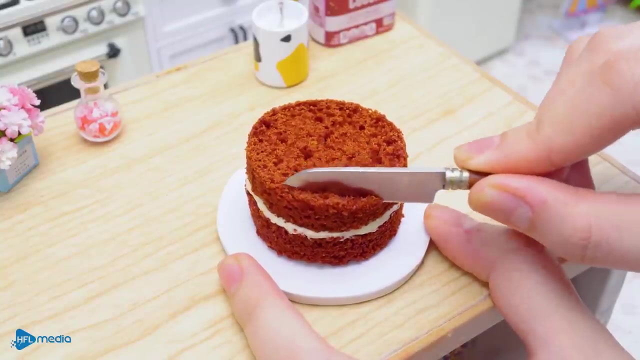 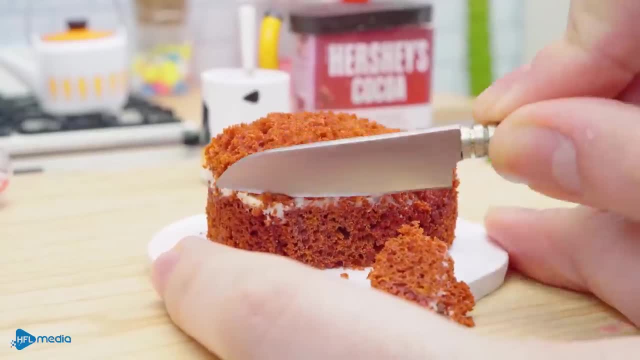 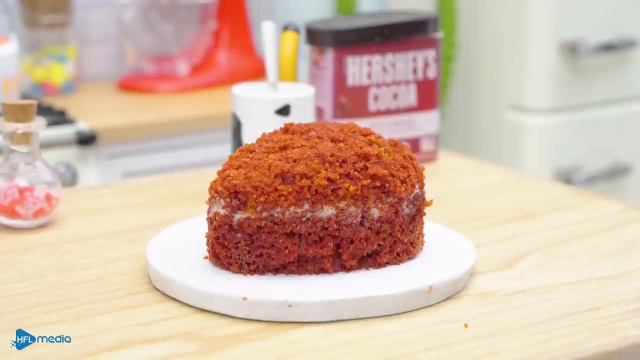 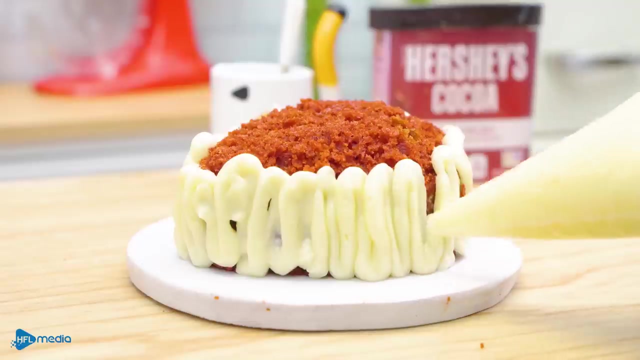 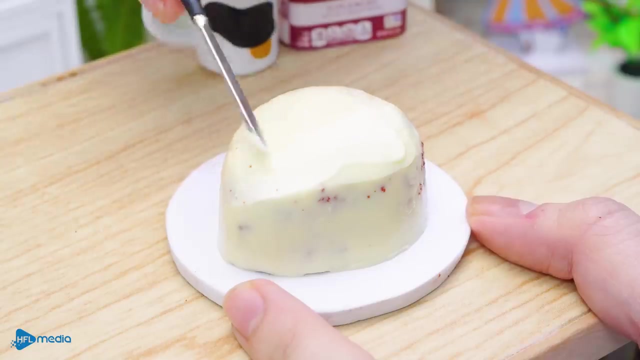 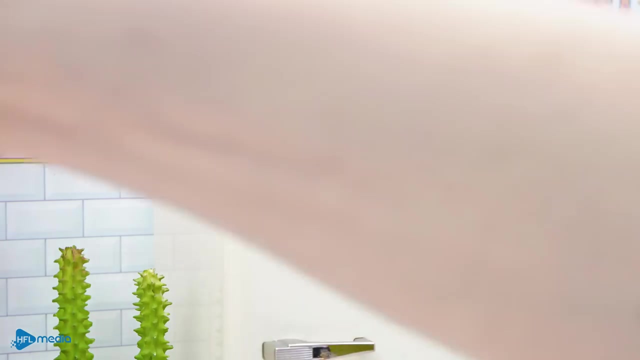 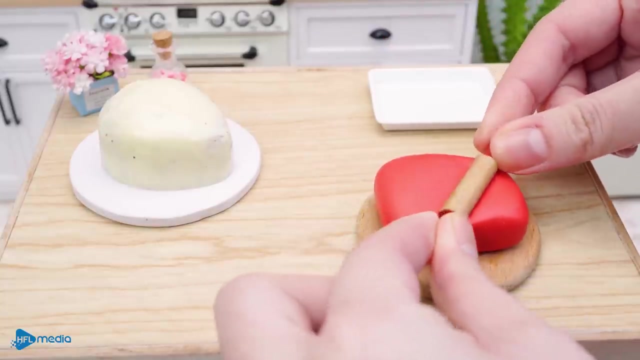 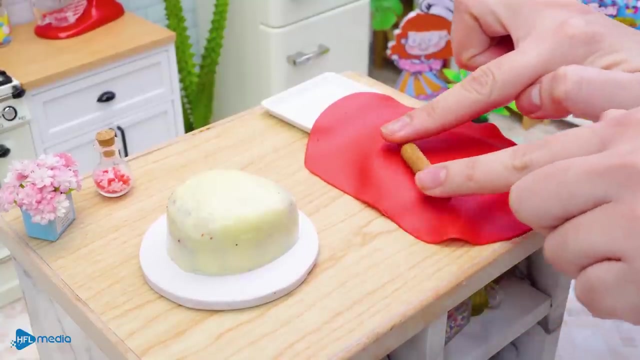 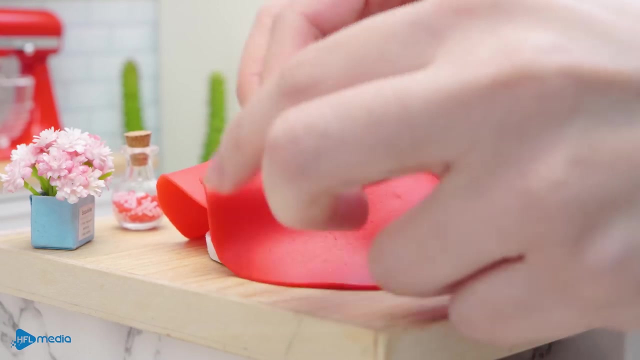 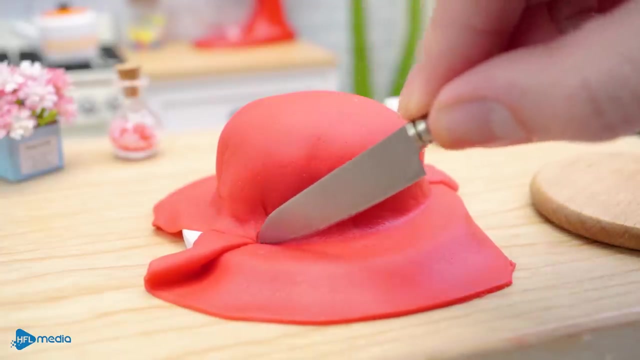 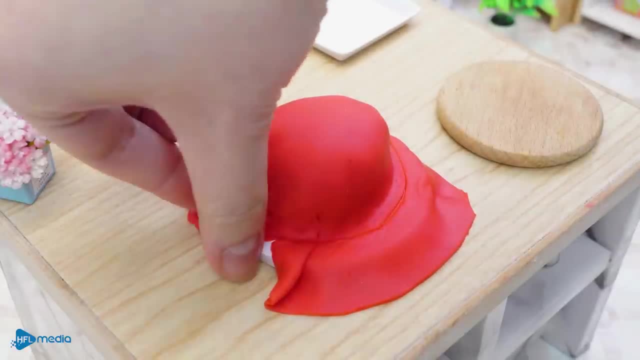 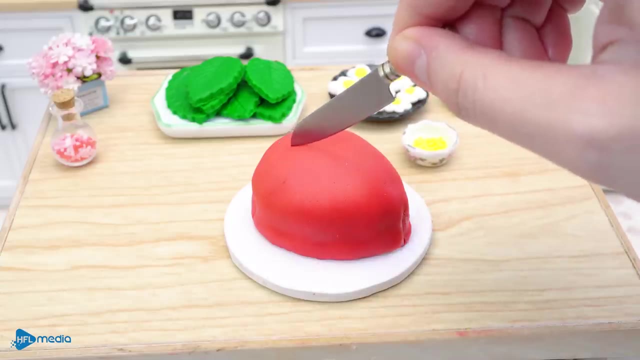 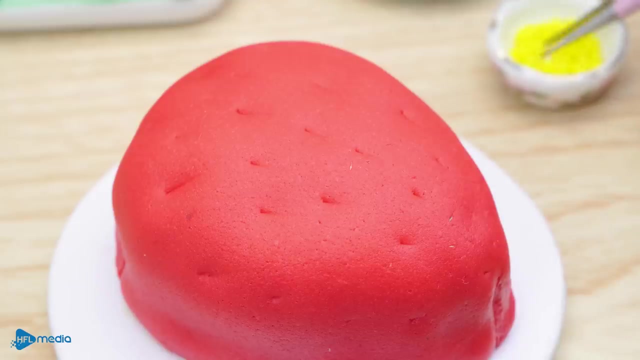 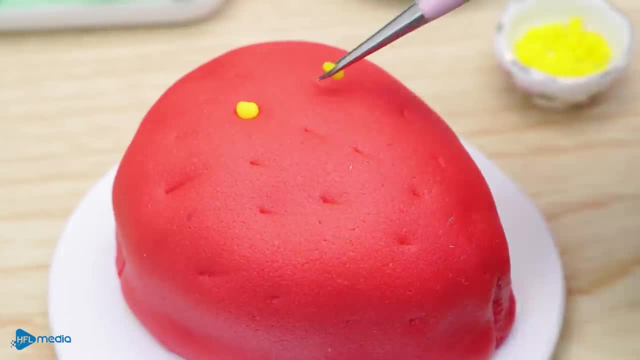 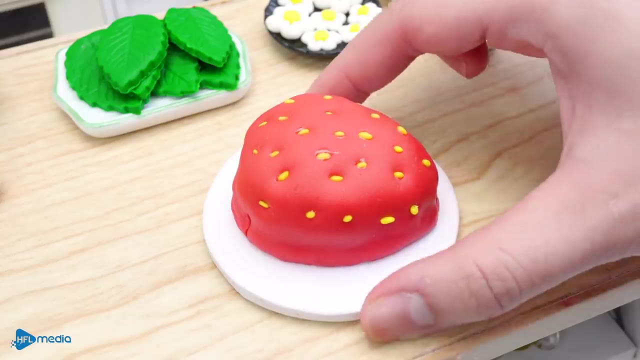 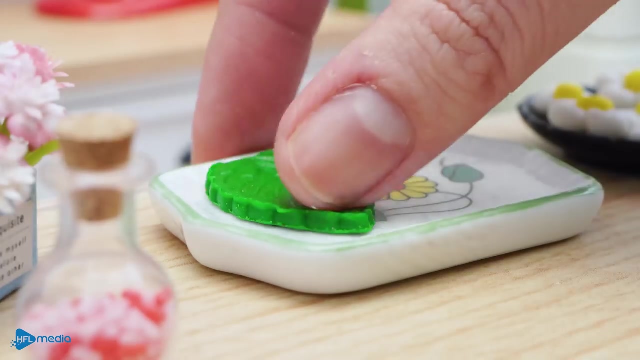 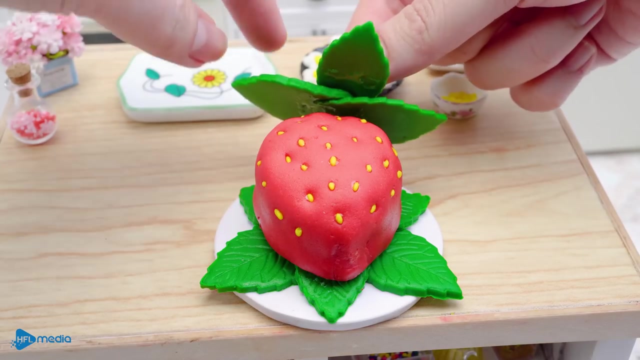 Cut it into bite-sized pieces to make it easier to eat. It's similar to watermelon. Let's小ør sfärő кориз. Make baklava Your favorite flavor, Then puta Lettuce governing. You. choose your favorite food color. I choose a이�ene. 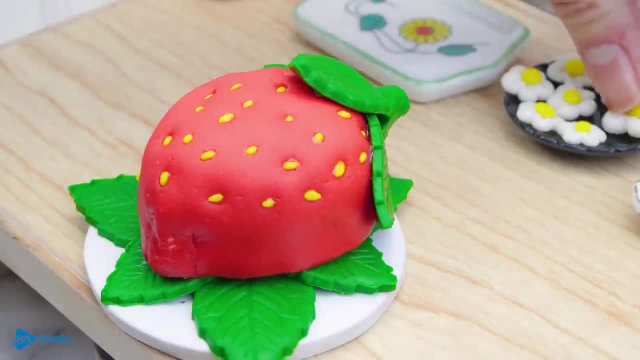 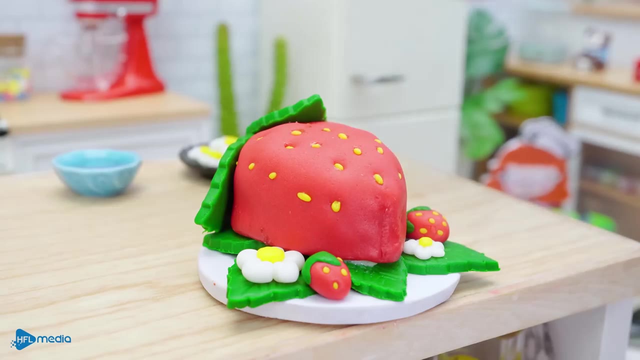 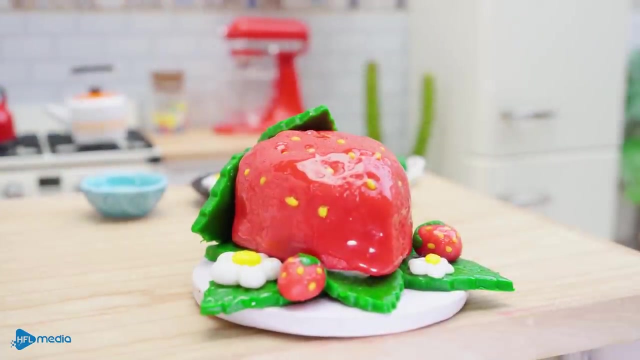 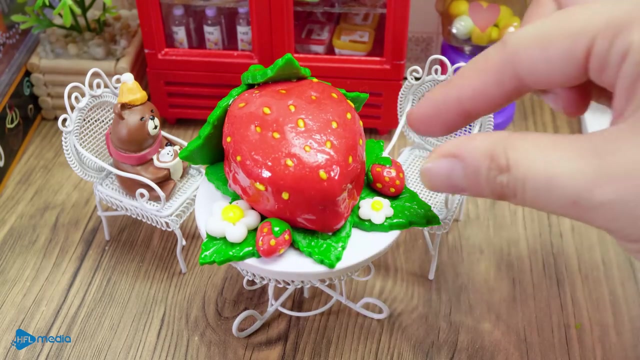 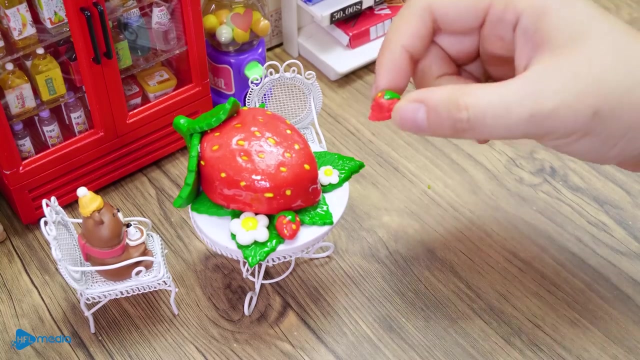 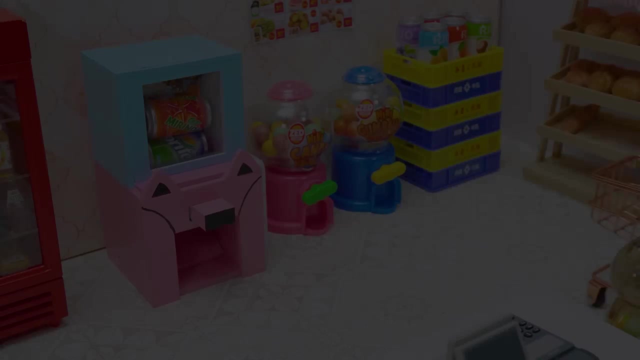 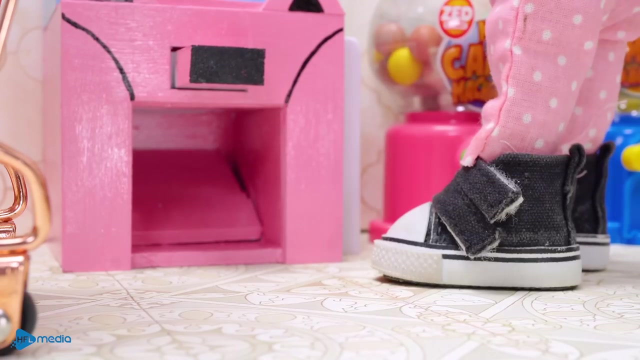 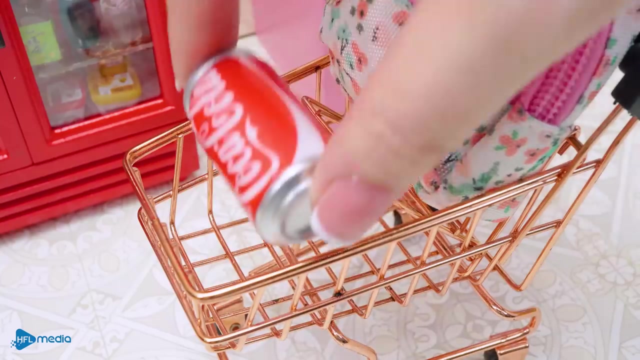 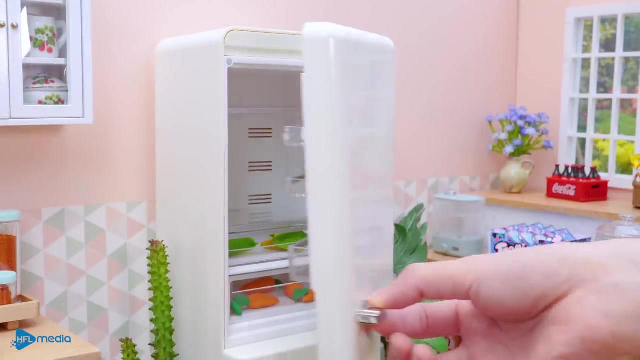 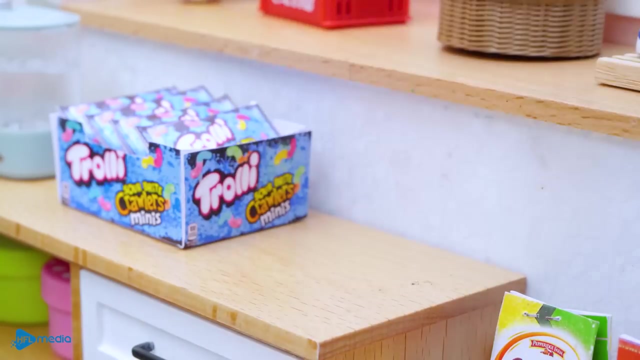 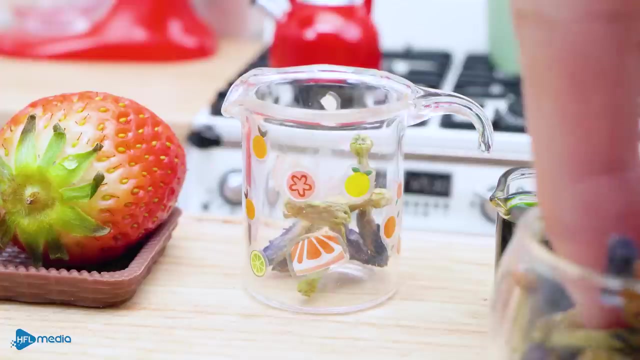 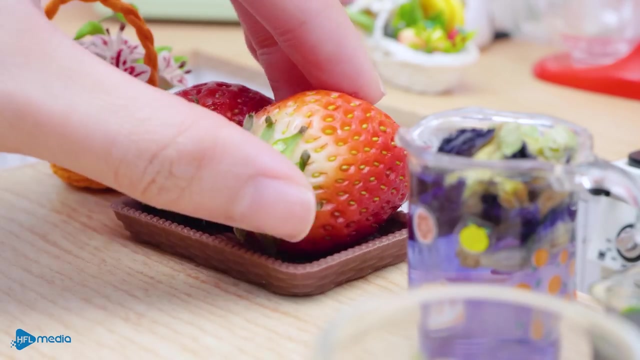 I choose a little bit of green and red. You choose your favorite food color. I cook simple without puta. I cook simple without puta applied. Ew, it tastes disgusting. Uh-huh, Hooray, Almost there, But still nothing. It's just so sweet. 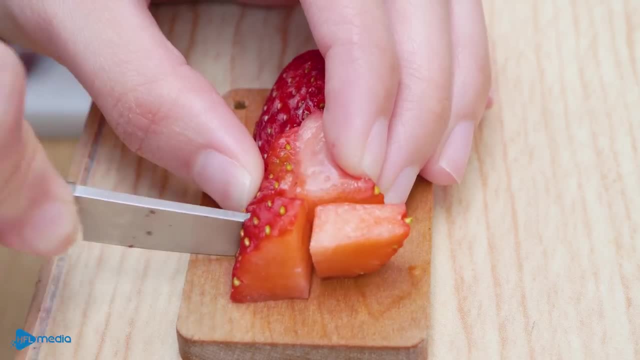 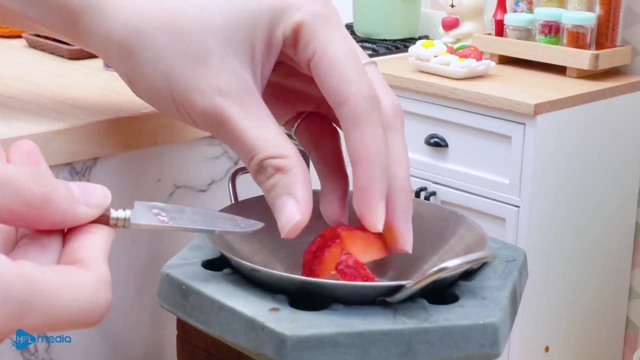 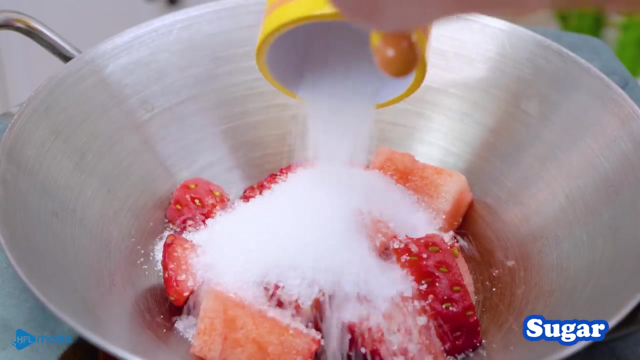 It's too sweet. We'll have to see where this kind of food goes. It's delicious. It's not my first time, But it's been a great experience. The taste is great. Soak in water for 30 minutes. If you want to eat it, you have to eat it right after it's cooked. 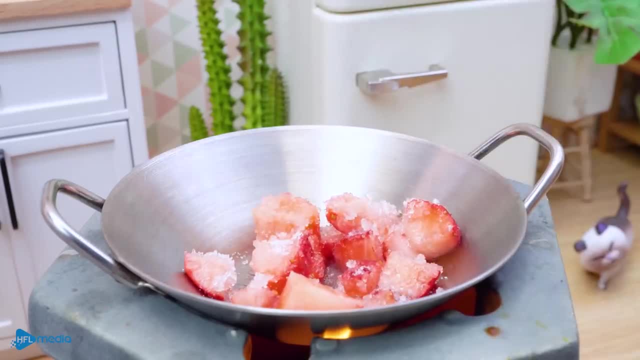 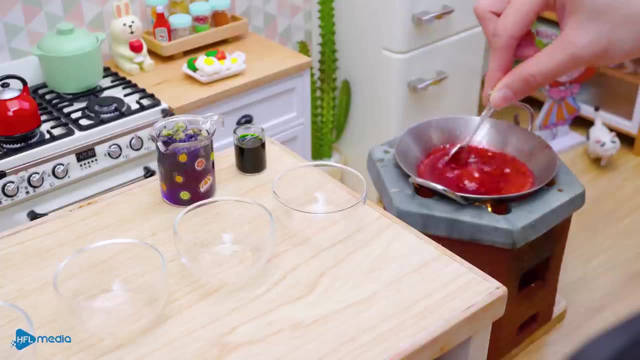 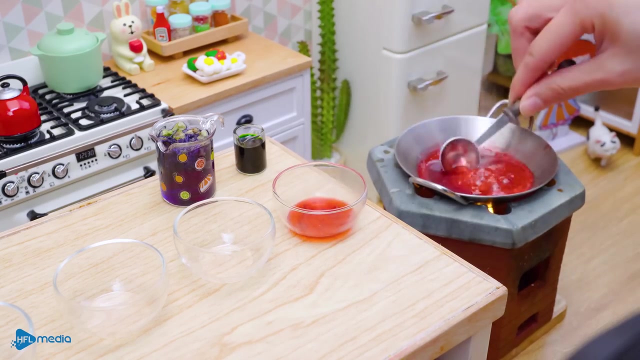 It's so good. This time I'll try it with a spoon. It's really good. It's really good. It's really good. It's so good, It's really good. It's so good, It's really good. 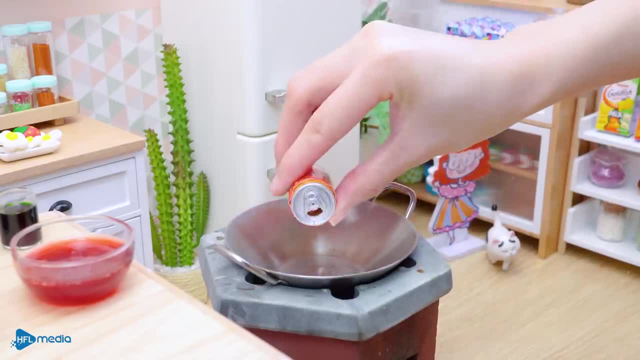 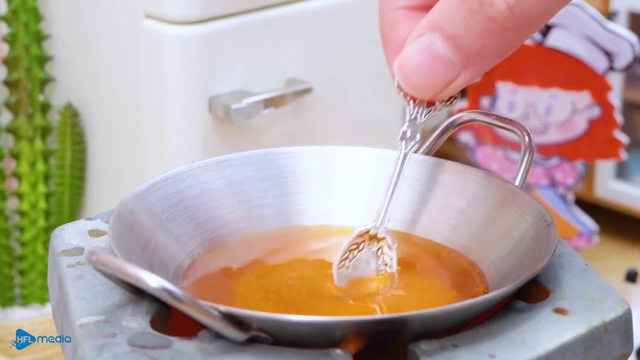 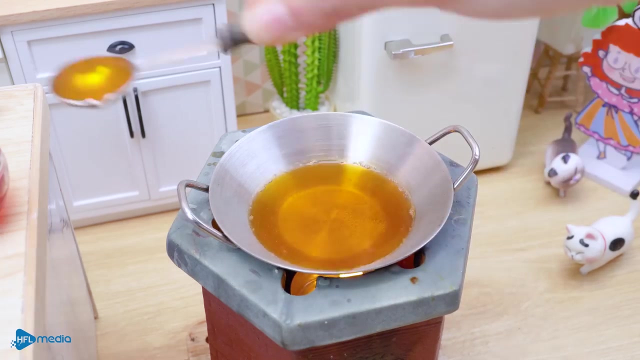 I'll try it with a spoon. It's really good. It's really good. Actually, I do this because if you're not interested in caregarding, I'm not even willing to go into detail about what these belong to. Let's get right into the english. 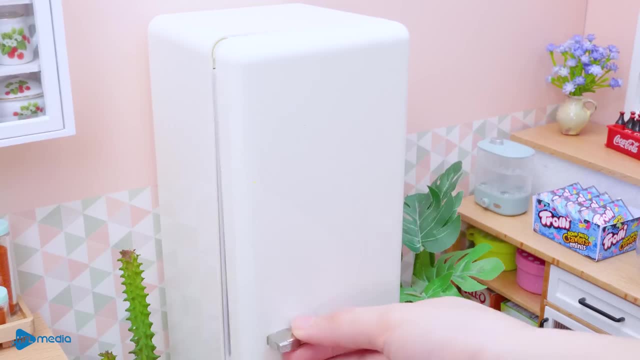 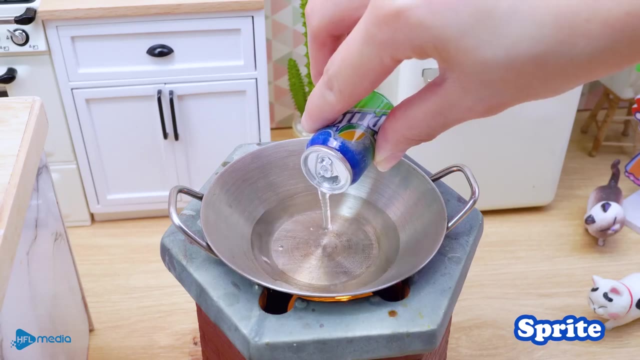 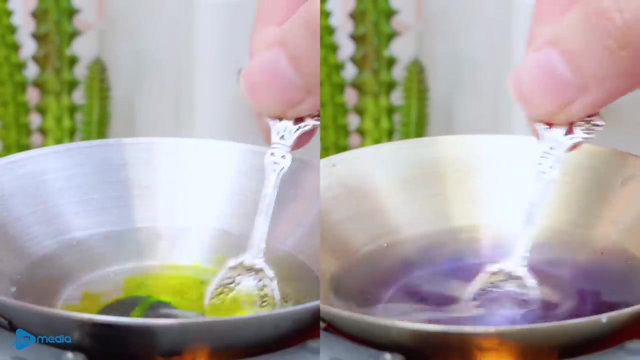 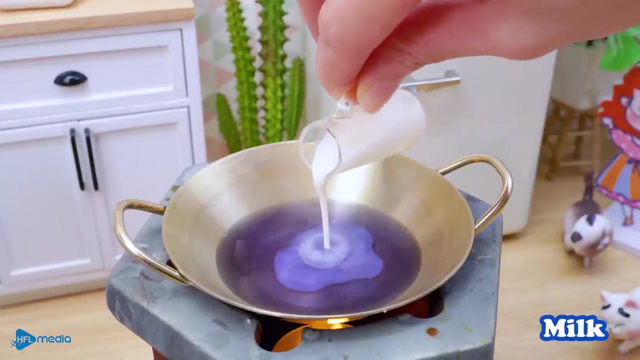 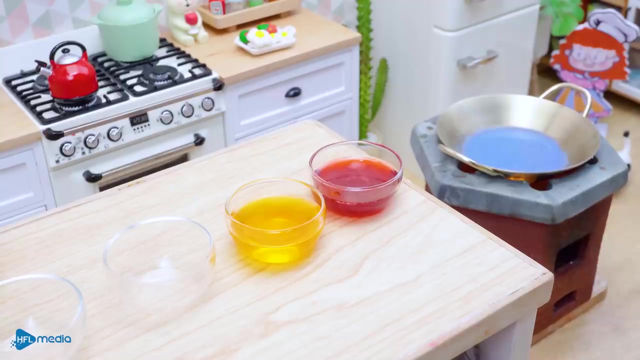 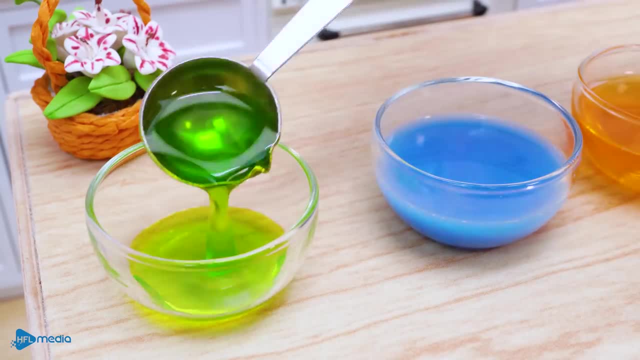 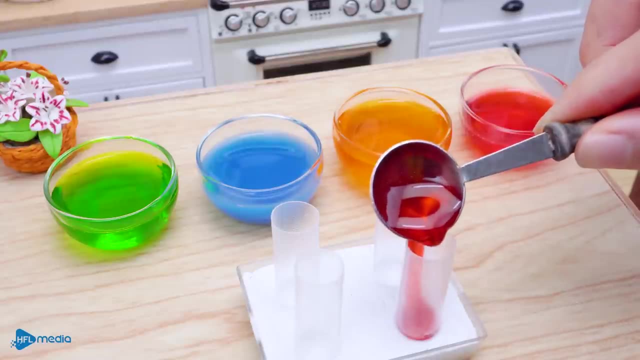 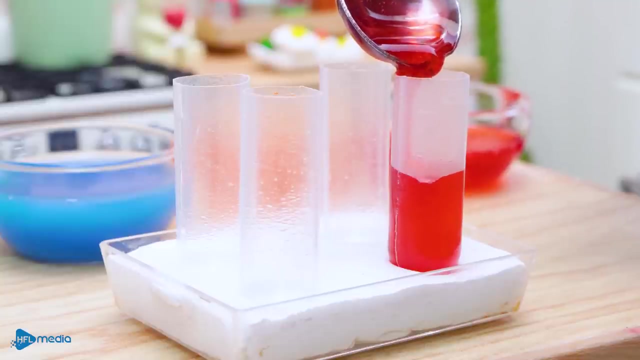 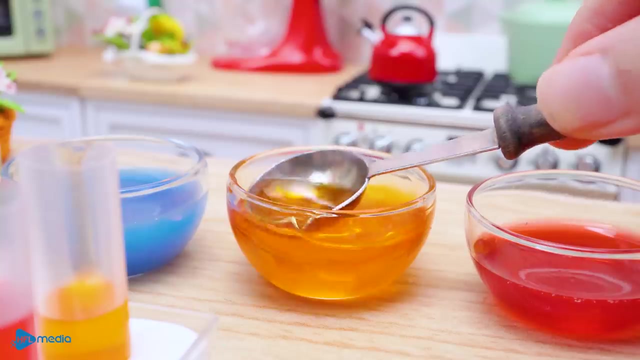 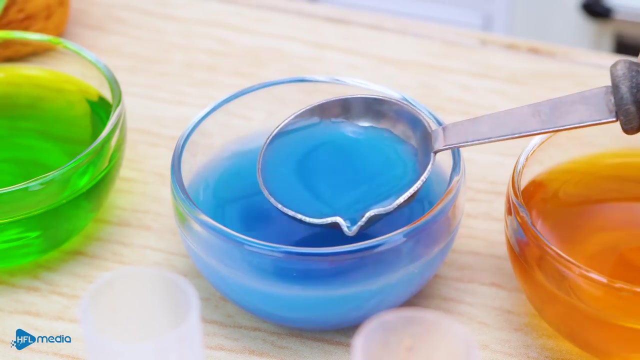 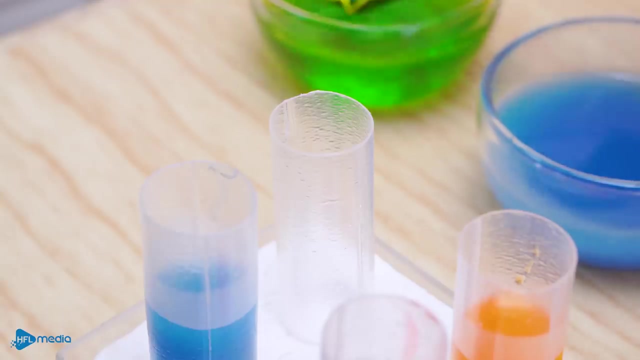 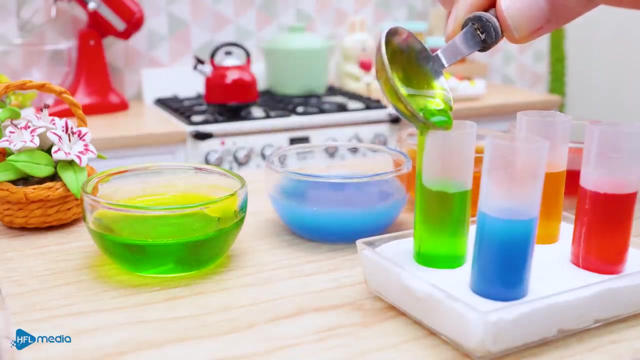 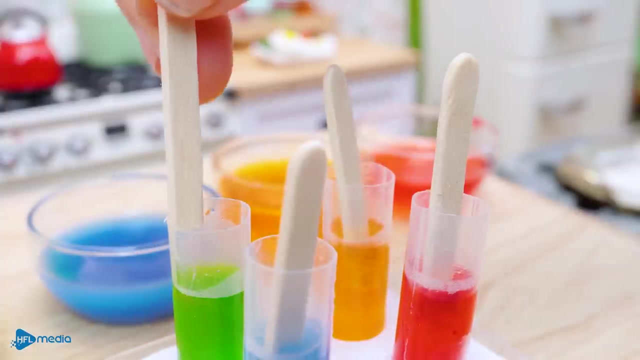 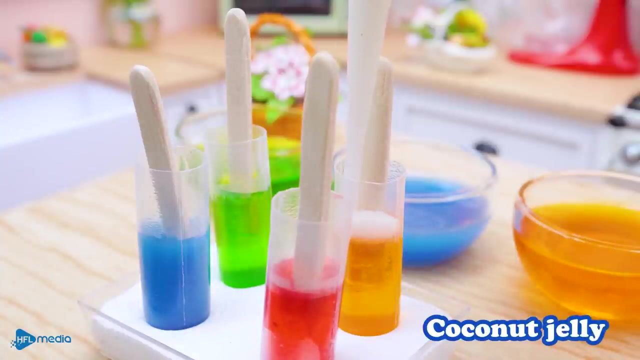 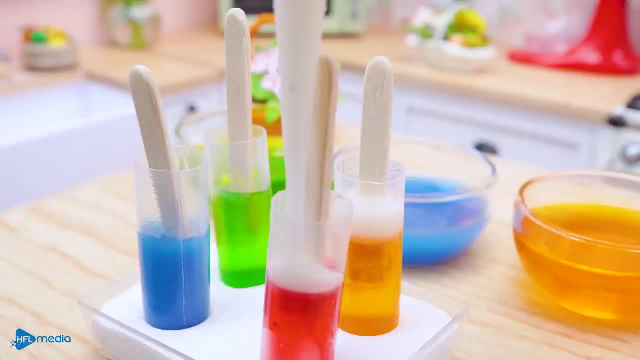 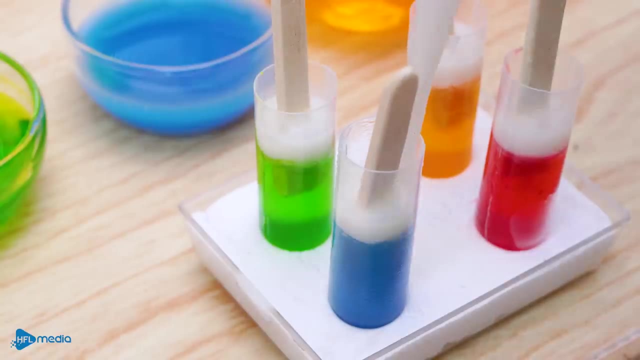 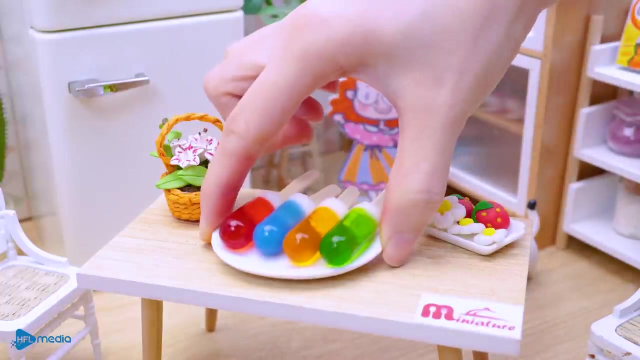 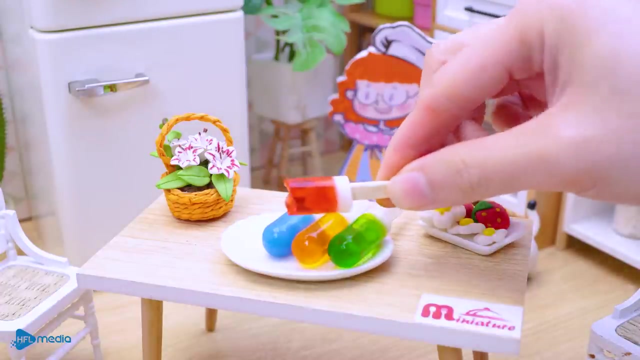 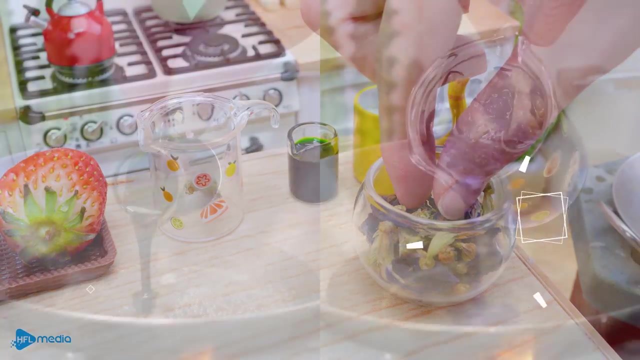 Mmm, really good. Thank you so much for watching my video today and I will see you in my next video. bye-bye.